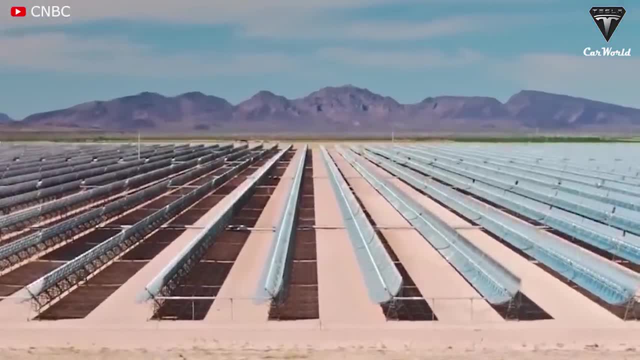 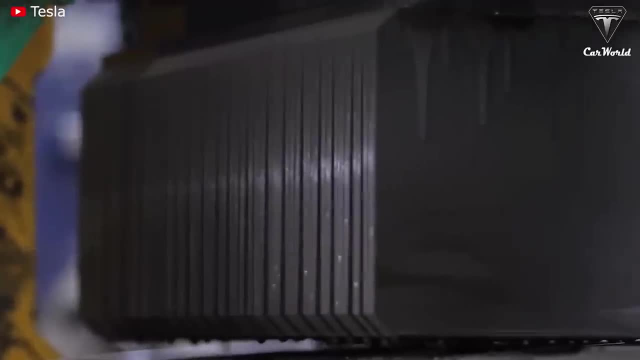 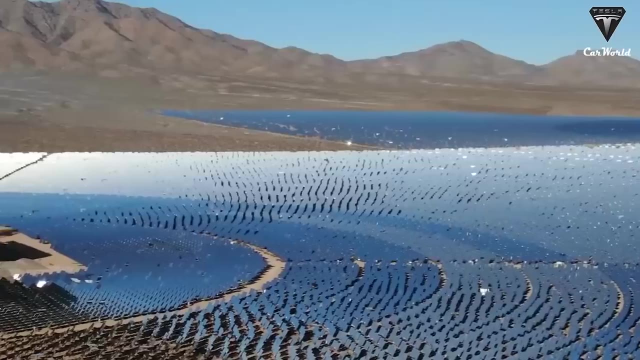 less and providing an endless flow of energy. As you know, the standard silicon photovoltaic solar cell is the black and copper solar panel that you can find on suburban rooftops and solar farms that were born and raised in America in 1950. Currently, 90% of the world's solar panels 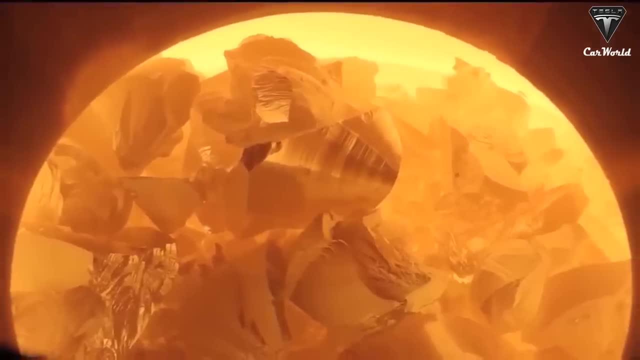 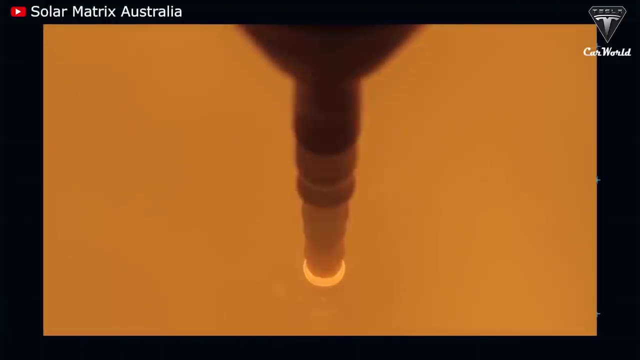 are made from crystalline silicon, and the industry continues to grow at a rate of about 30% per year. Now, what have we told you about a material that is lighter and simpler to manufacture at a lower cost. It's an inexpensive solution that can make 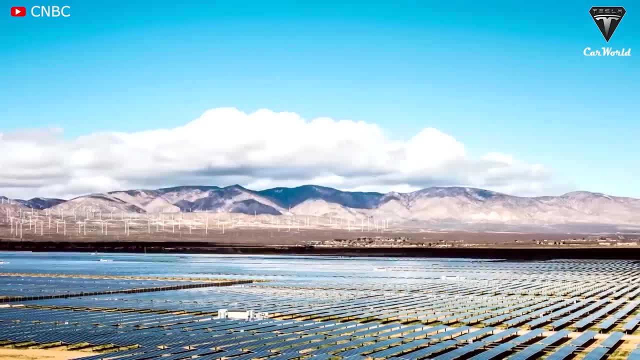 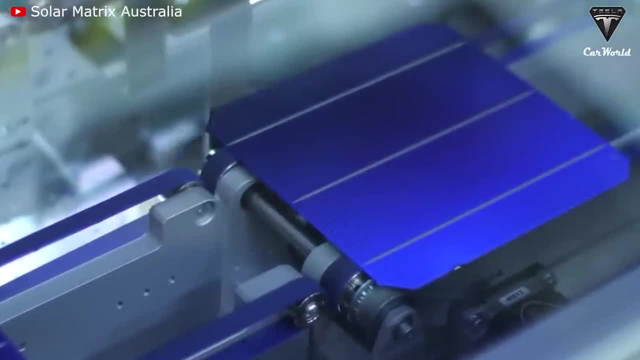 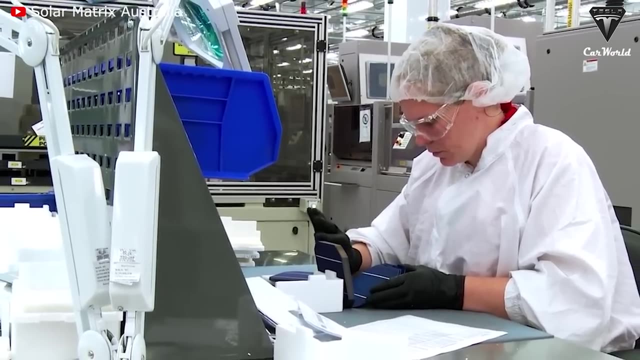 an amazing living. If you're interested in learning more about solar panels, you can click on the link in the description. These photovoltaic cells thin enough to power a house are called ferroelectric crystal cells. Strong demand coupled with production glitches has pushed the price of key materials, mainly polysilicon, for solar panels to the highest. level. The cost of the most expensive grade of polysilicon rose to $40.62 per kilogram, surpassing last year's high of $40.34.. Polysilicon is a very expensive material but it's worth the money. Polysilicon makers take the 99% pure silicon metal and remove impurities. 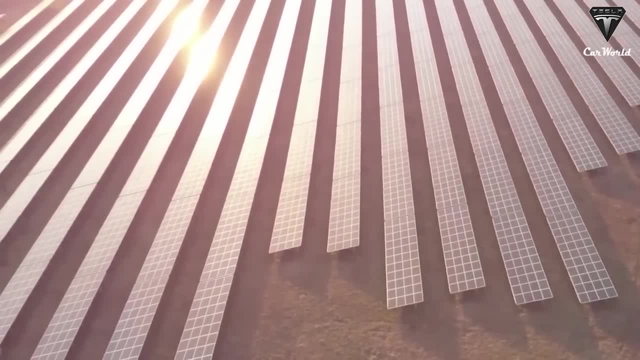 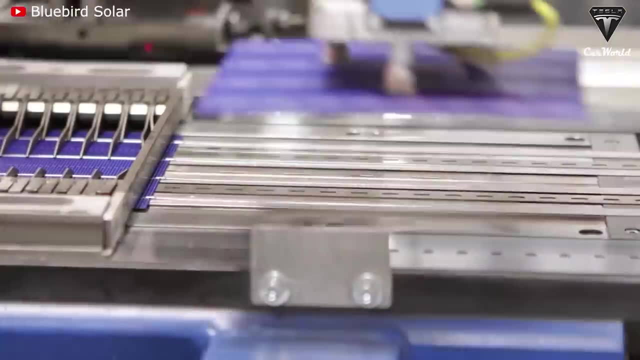 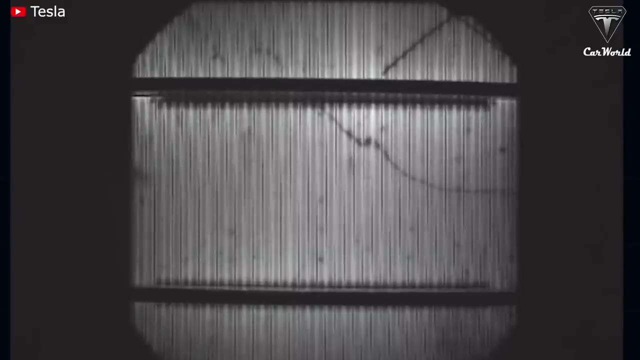 until it is 99.9999% pure. As the silicon rods are forming at the center of the reactor, the reactor walls need to be kept cool to prevent the silicon from crystallizing there. Maintaining that temperature difference is really energy intensive. 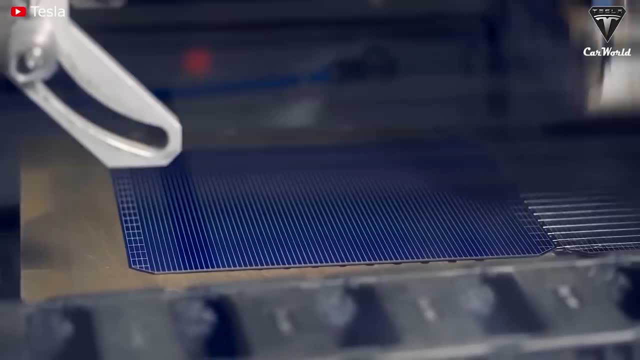 prompting Tesla to find an alternative to silicon. The energy generation of ferroelectric crystals in solar panels is a very important part of the process. The silicon is a very important part of the process. The silicon is a very important part of the process. The silicon is a very important part of the process. 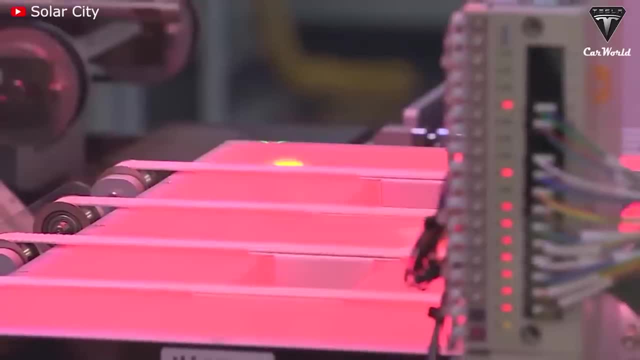 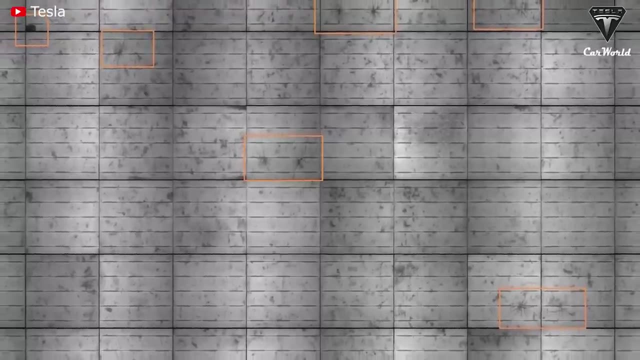 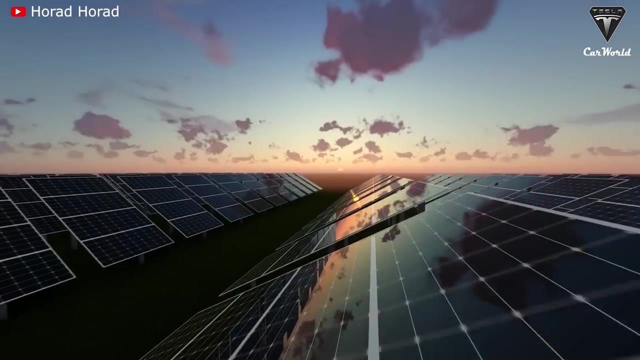 Solar cells can be increased by a factor of a thousand thanks to a new innovation involving the arrangement of thin layers of the materials. Ferroelectric crystals differ from conventional silicon cells in that they do not require a p-n junction to create the p-v effect. In other words, 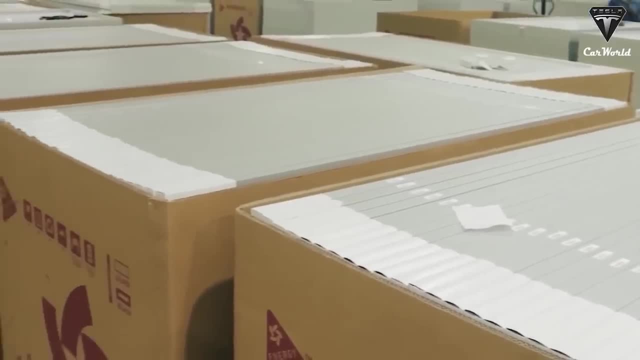 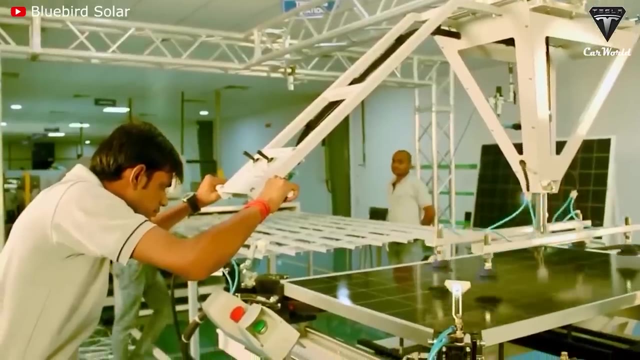 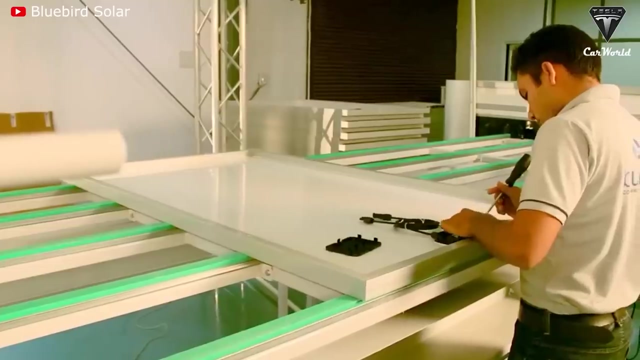 there is no need to create positively and negatively doped layers within the cell. The researchers said that change could make solar panels easier to produce. Raw materials for the production of this new cell do not need to be mined from the earth. It is any material with a. 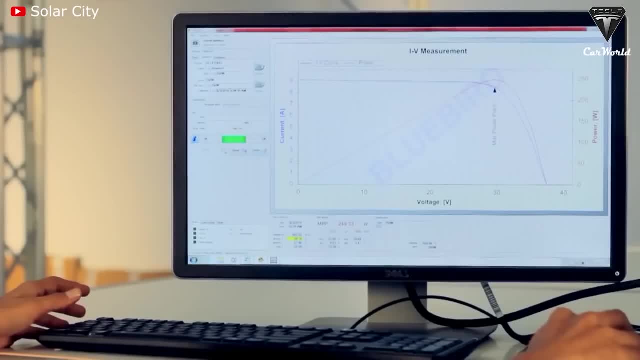 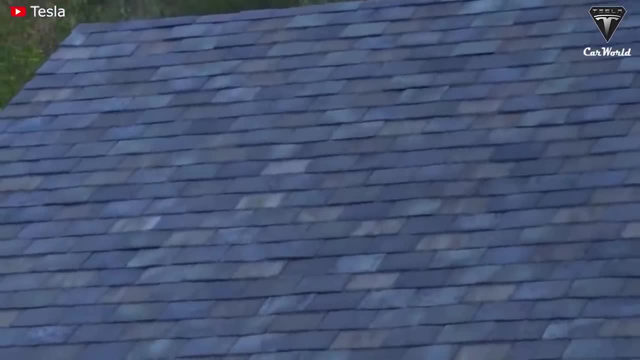 crystalline structure. so researchers use ferroelectrics like barium titanate, a mixed oxide made of barium and titanium. This significantly reduces costs. Tesla does not need to invest a lot of money in professional workers or high-tech machinery to support the 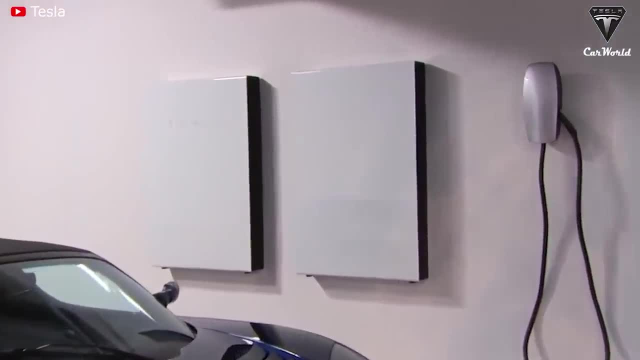 production. Therefore, it's estimated that these panels can cost up to 10 times less per watt than modern commercial silicon. Tesla does not need to invest a lot of money in professional workers or high-tech machinery to support the production of silicon solar panels. You can expect to pay. about $2.21 per watt for Tesla's solar panels before the federal solar tax credit, but this ferroelectric panel only costs $0.22 per watt. Previously, you always had to worry about the price of silicon solar panels, while this new Tesla innovation is a great solution for those who 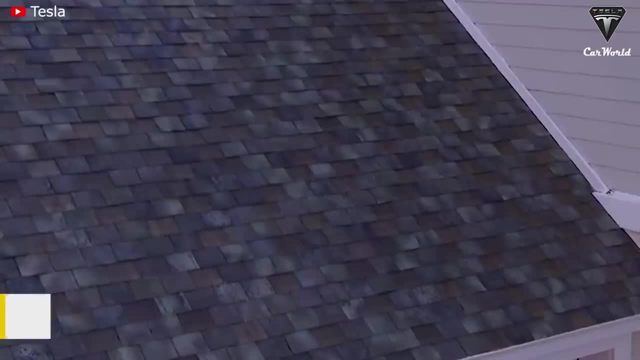 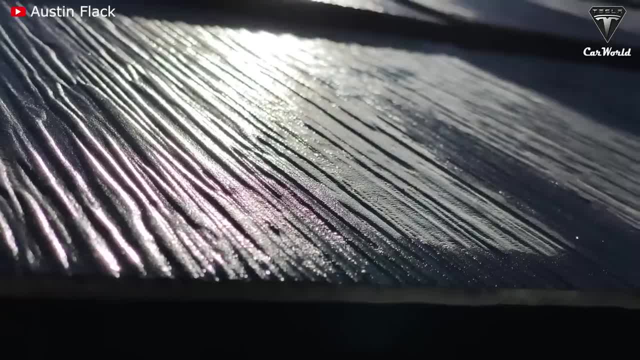 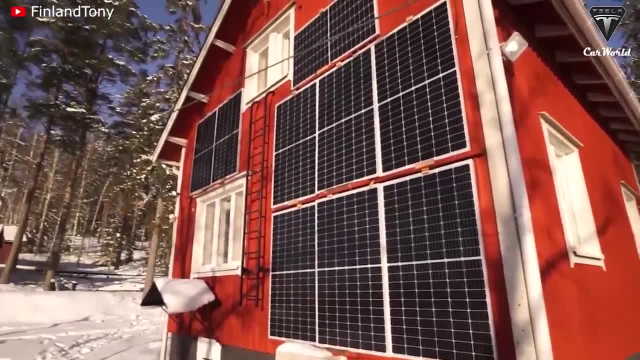 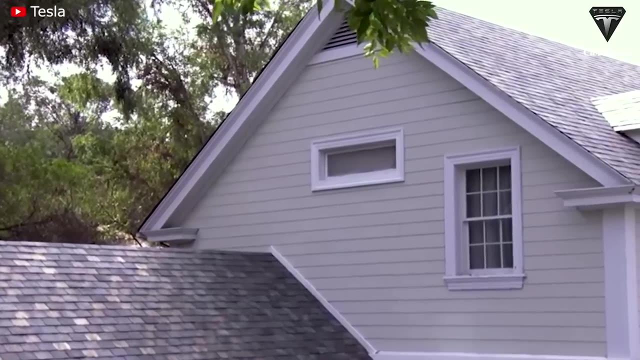 The US installed 3.9 gigawatts of solar PV capacity in the first quarter of 2022, to reach 126.1 gigawatts direct current of total installed capacity- enough to power 22 million American homes. Solar accounted for 50% of all new electricity generating capacity added in the US in the first quarter. Elon Musk said Tesla's new cell will change the game because it can generate more energy than ever before. The US installed 3.9 gigawatts of solar PV capacity in the first quarter. Elon Musk said Tesla's new cell will generate more energy than ever before. 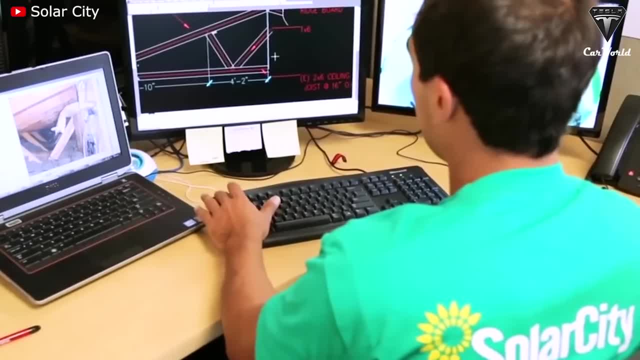 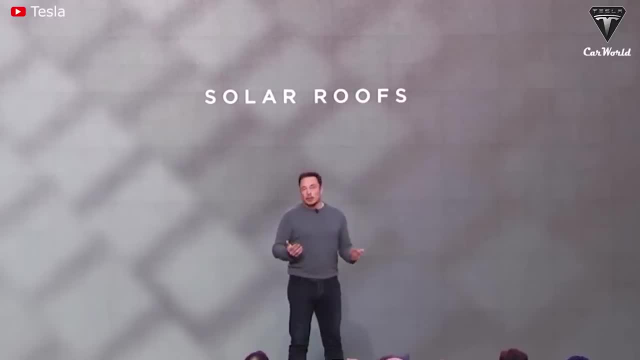 To achieve this increase in electrical energy production, the researchers created crystalline layers of barium titanate, strontium titanate and calcium titanate, which they placed alternatively on top of one another, separating the positive and negative charges in the same photovoltaic. 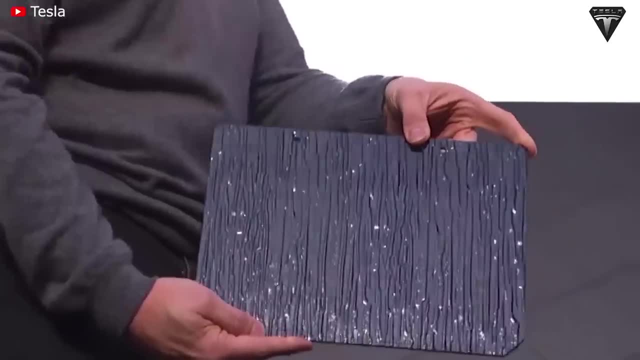 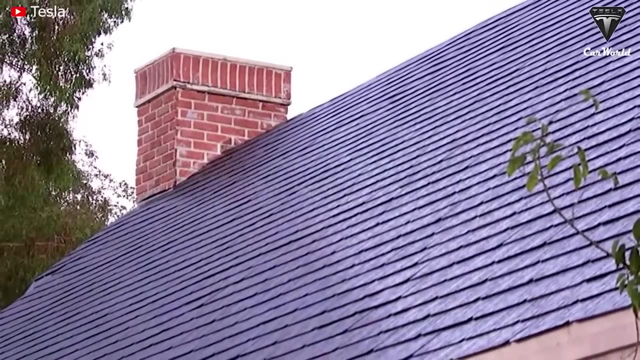 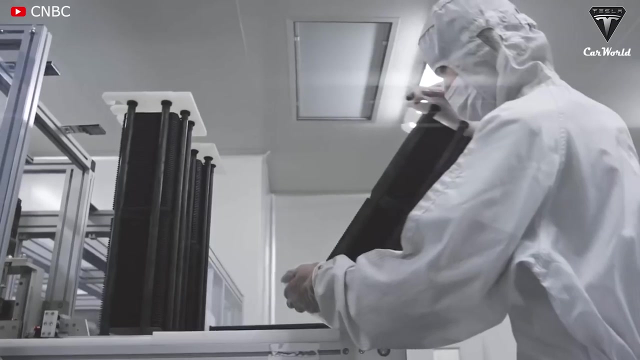 device. This arrangement could greatly increase the efficiency of solar panels. However, pure barium titanate, a ferroelectric crystal, does not absorb much sunlight and consequently generates a comparatively low photocurrent. The researchers discovered that combining extremely thin layers of different materials significantly increases the solar energy yield. 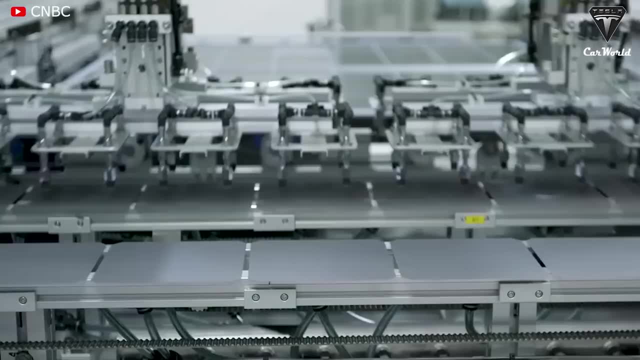 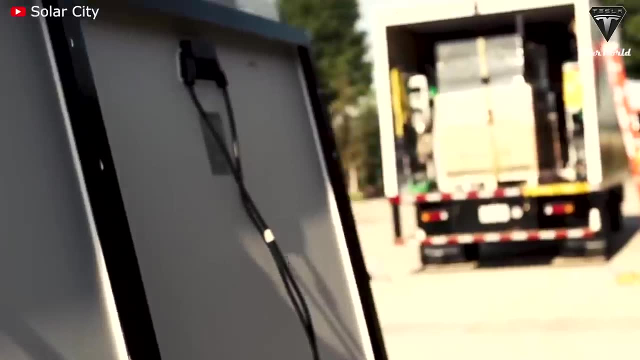 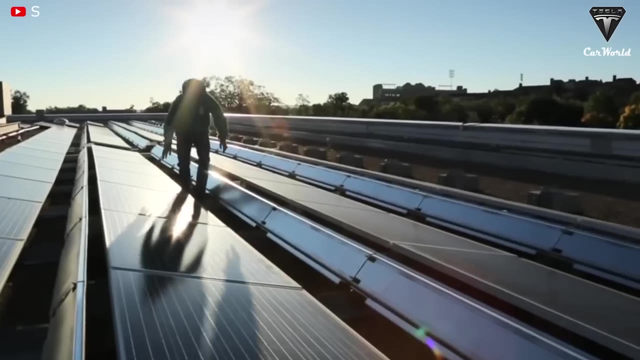 by experimenting with different material combinations. This was achieved by vaporizing the crystals with a high-power laser and redepositing them on carrier substrates. This produced a material made of 500 layers that are about 200 nanometers thick In comparison with. 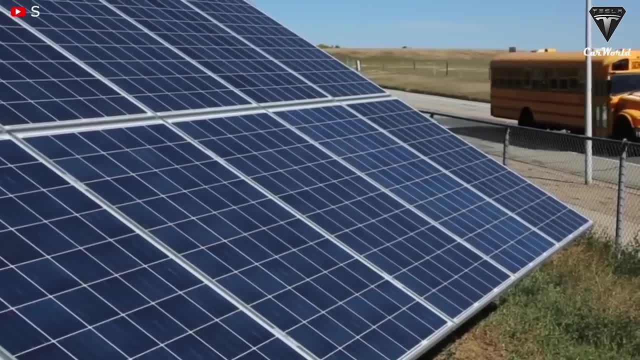 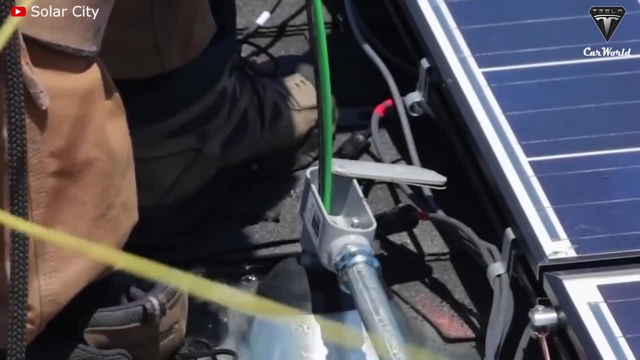 pure barium titanate. the solar energy yield of the solar panels is about 200 nanometers thick. In comparison with barium titanate, the new photoelectric material irradiated with laser light had a current flow 1,000 times stronger and more efficient, even with a reduction. 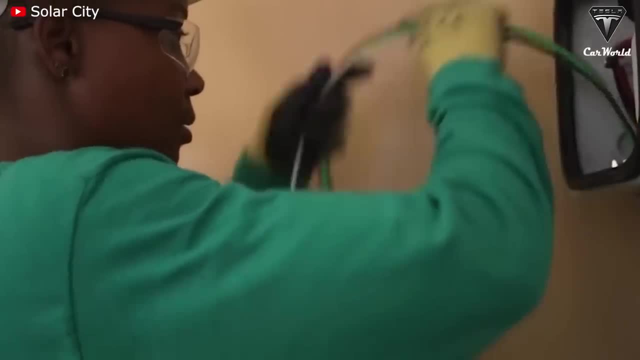 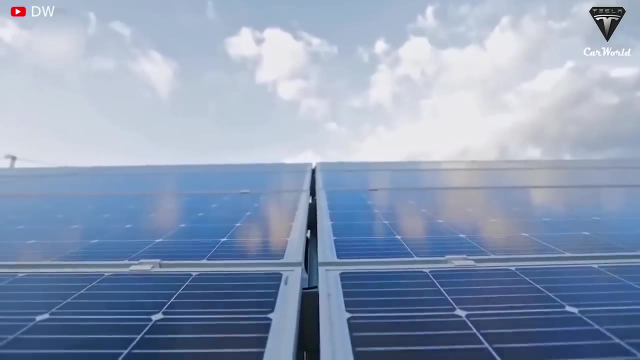 in the proportion of the base element of the mixture by almost two-thirds. The interaction between the lattice layers appears to lead to a much higher permittivity. In other words, the electrons are able to flow much more easily due to the excitation by the light photons. 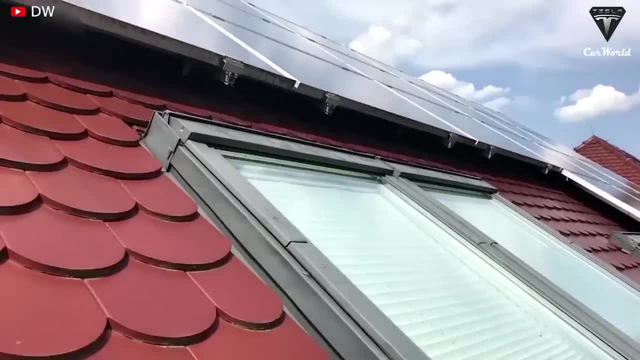 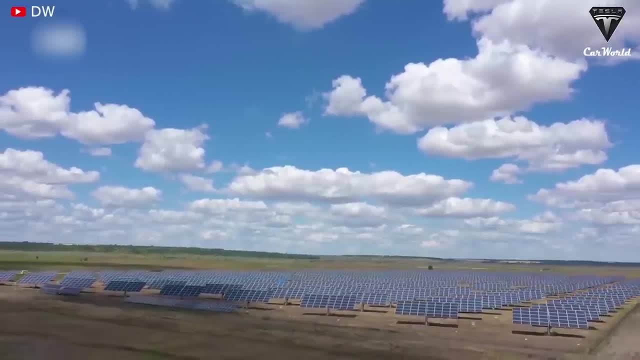 The measurements also showed that this effect is very robust. It remains to be seen how this effect will affect solar panels. A large Tesla solar system of 11.34 kilowatts can produce an average of 43 to 58 kilowatt hours per. 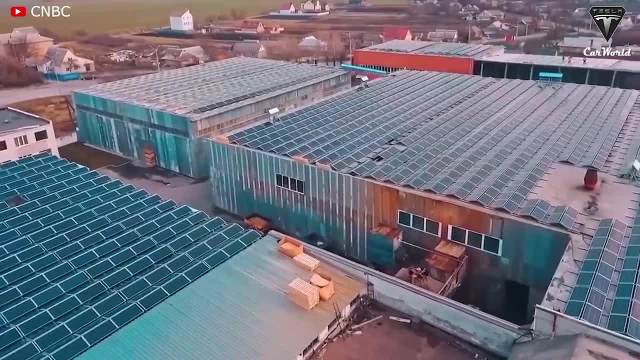 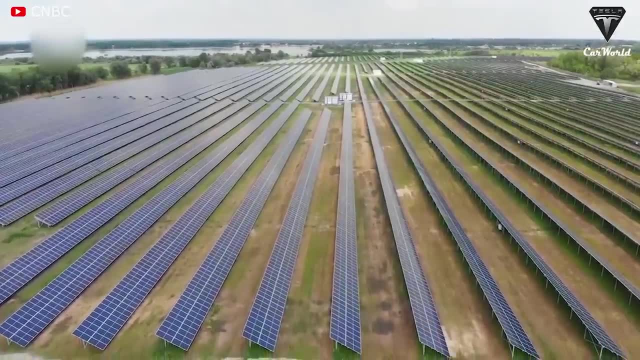 day, equivalent to 1,500 kilowatt hours per week With a ferroelectric cell. don't be surprised when we say that it can produce 1.5 million kilowatt hours per week. The ferroelectric cell development. 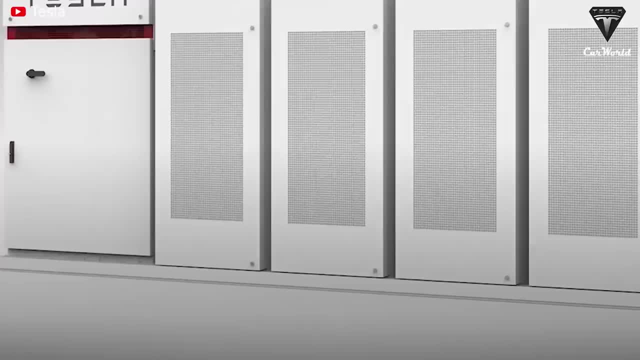 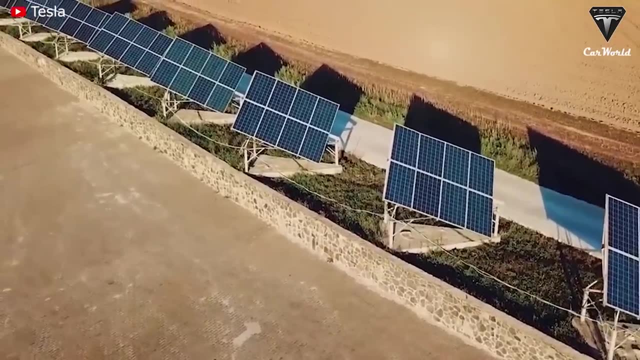 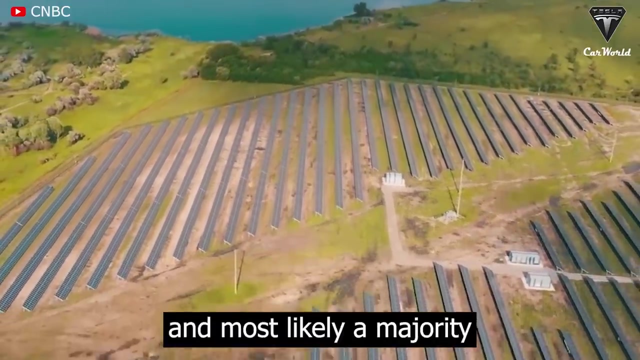 plan is a big step forward for Tesla as well as the renewable energy market. In the future, this cell is predicted to fulfill Elon Musk's ambition to provide electricity for the entire United States. Elon Musk's prediction is also a big turning point for the United States. 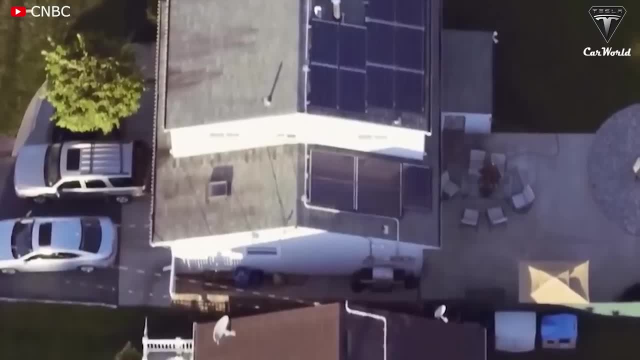 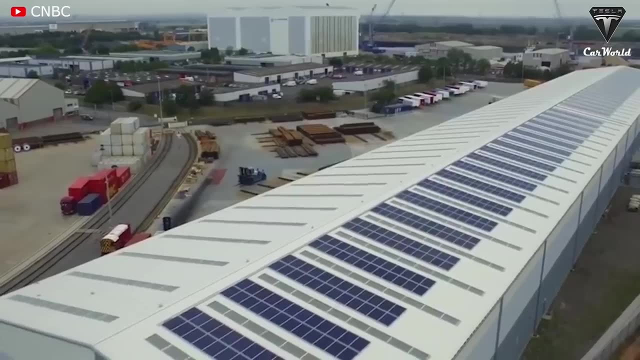 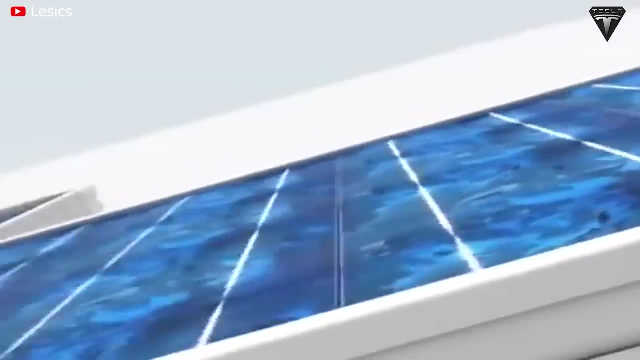 A future with more solar energy could open the door to many different use cases. You can integrate those panels into public transport on the road in your Model Y and imagine buildings covered with transparent windows at job-free. Thanks for watching- generate electricity. How exciting. So what are the challenges for ferroelectric solar cells? 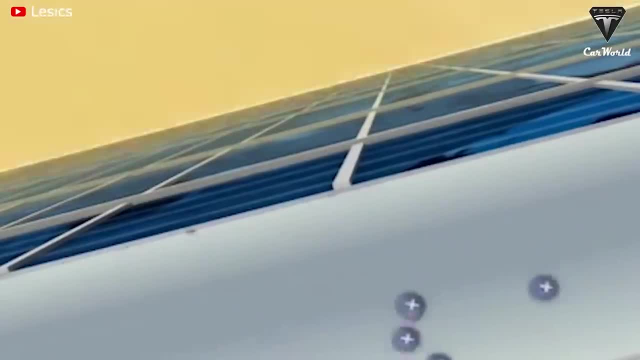 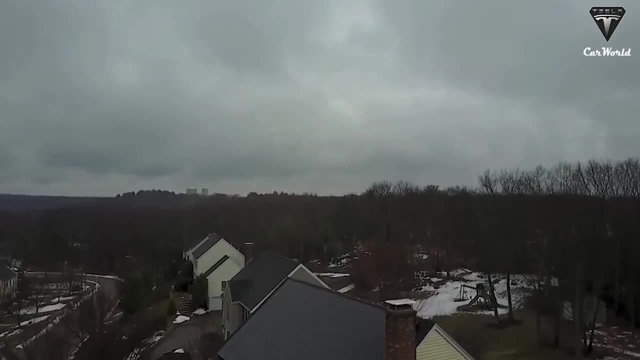 A common problem with thin films is that high temperatures shorten lifespan. For the western states, silicon crystal holds the best position so far. Tesla is working on creating a thin film that can withstand extreme temperatures. Their work promises to be part of a potential revolution. 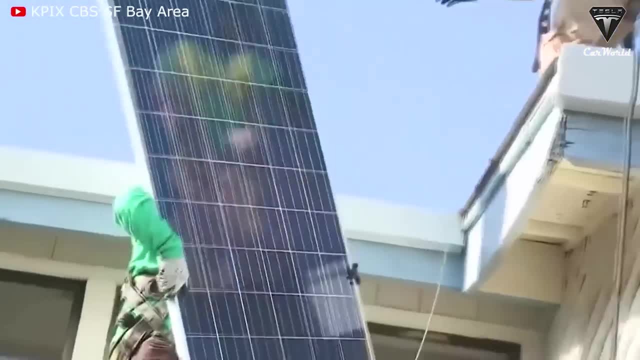 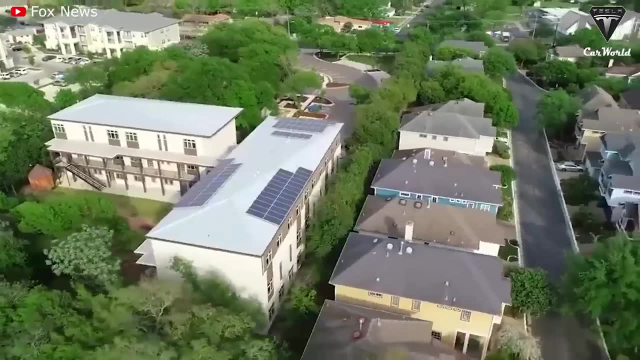 in ferroelectric materials, with possible applications in computer memory capacitors and other electronic devices. A silicon solar panel can last for 25 years. On the other hand, this ferroelectric cell is relatively new and needs time to be studied in the lab. 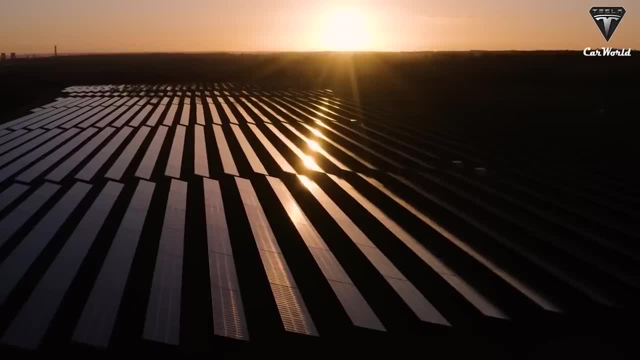 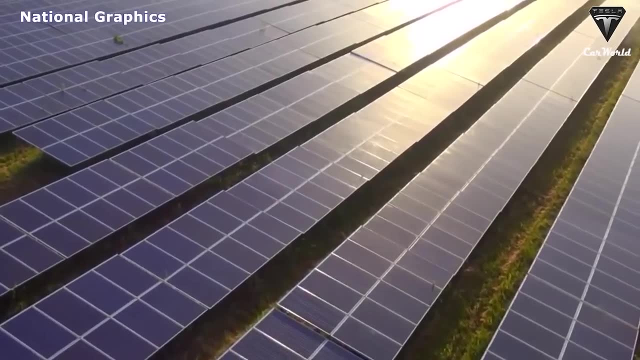 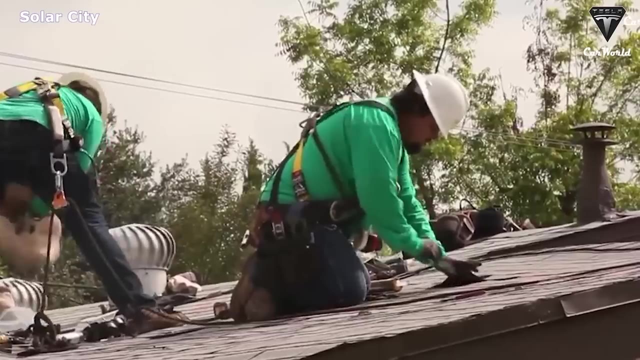 US President Biden has launched a series of initiatives to spur domestic solar PV manufacturing with 56 million US dollars in new funding. Solar technology is accelerating at such a fast pace that it makes us wonder what kind of stuff they'll be making 10 to 20 years down the road. 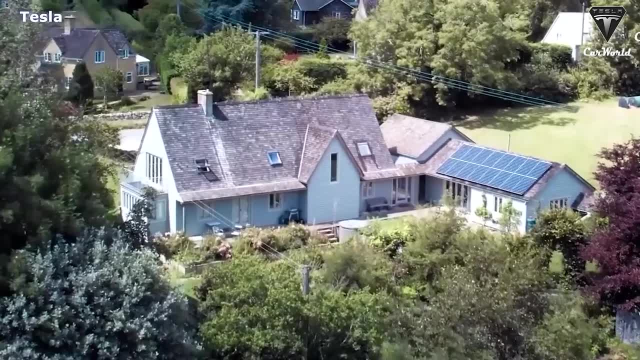 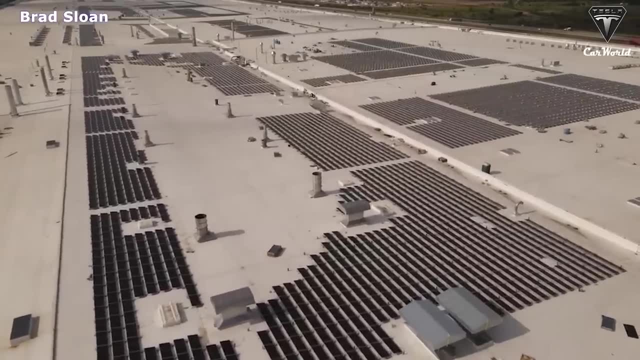 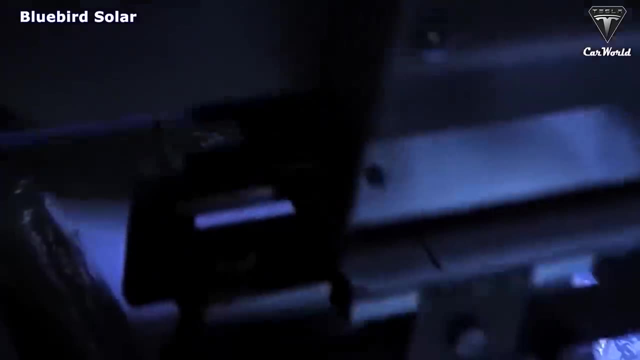 If you're thinking about buying solar panels but you don't want to remove your dome roof, then flexible solar is an interesting option. So does it have a chance to break away from the traditional rectangular glass panels? The future of solar technology extends far beyond. 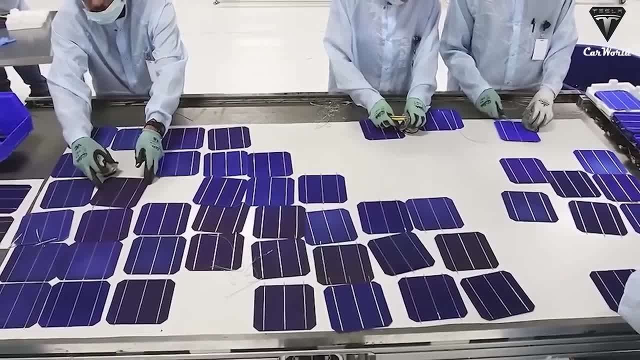 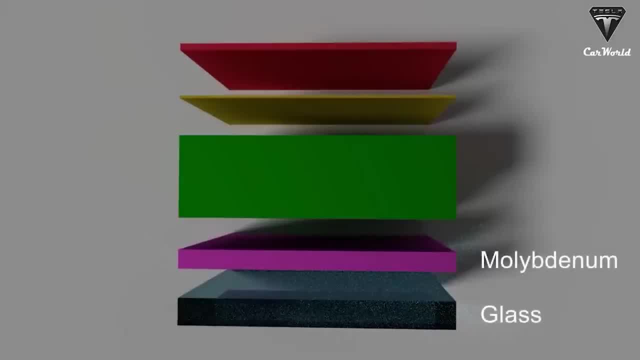 silicon with numerous alternative materials that belong to a certain class called thin film. Among various materials for thin film, solar cells, copper, indium gallium selenide is one of the most developed, having achieved efficiencies rivaling those of crystalline silicon. 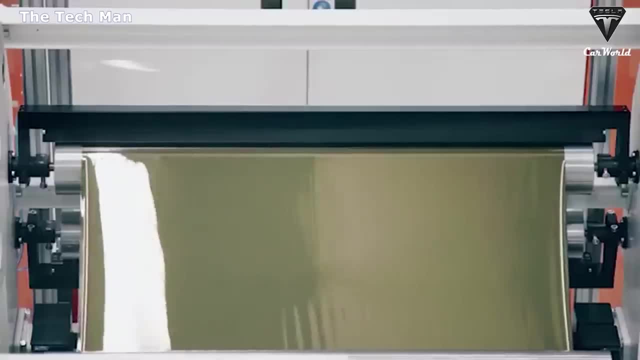 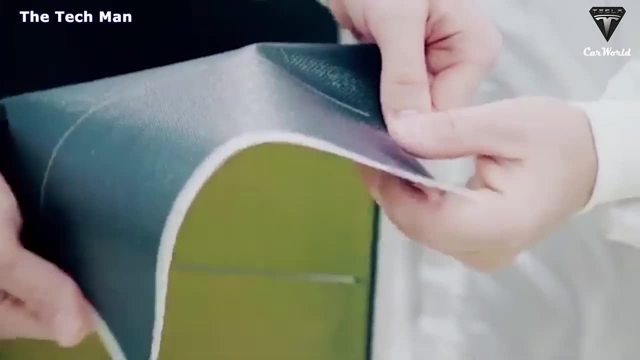 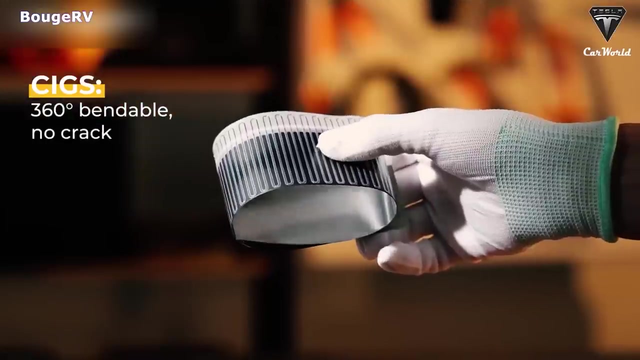 Though commercial manufacturing of CIGS solar products has faltered in recent years, the technology has retained plenty of interest among researchers, particularly for its potential in flexible or multi-junction devices. Bouge RV recently released its new copper indium gallium selenide thin film solar panel that has been gaining praise from users and experts alike. 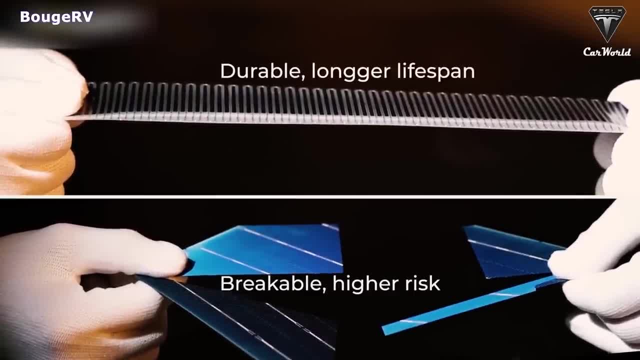 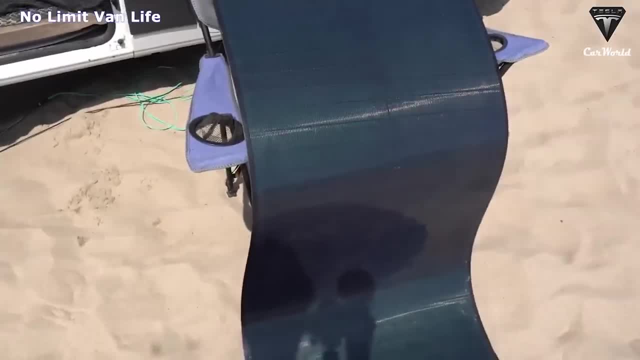 The new material in this solar panel is a new type of solar panel that is being developed in the field of solar energy. The new material in this solar panel can be a supplement to existing solar panels. Not only that, it's the company's first go at it. The new flexible solar cell is a thin-film. 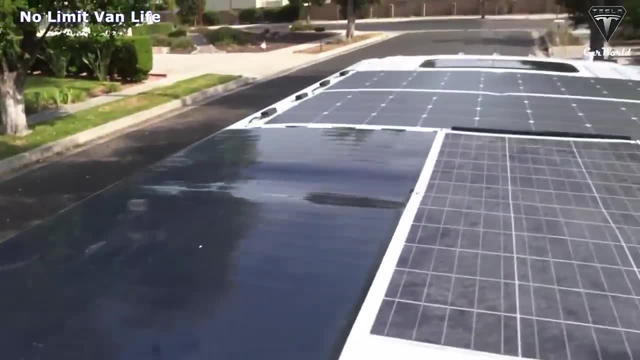 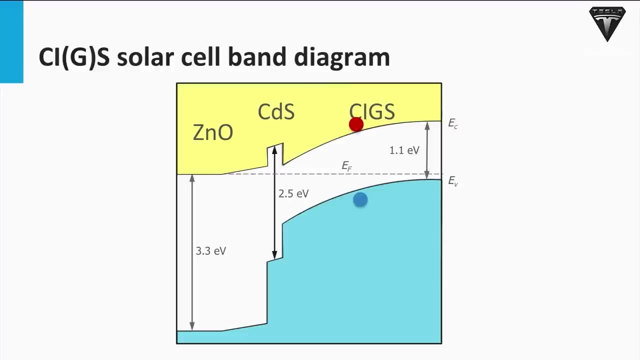 photovoltaic device that absorbs sunlight and converts it into electricity. It's created with CIGS and cadmium sulfide, for the absorber generates power by absorbing photons from incoming sunlight and then producing electrons that travel from the N-side to the P-side or negative side to the positive side of the junction. The solar panel is a new type of solar panel that will be produced by a company called GAS, which is a new type of solar cell that will be produced by a company called GAS, which is a new type of solar cell that will be produced by a company called. 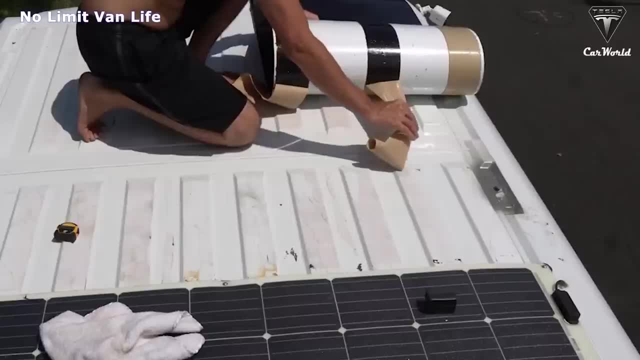 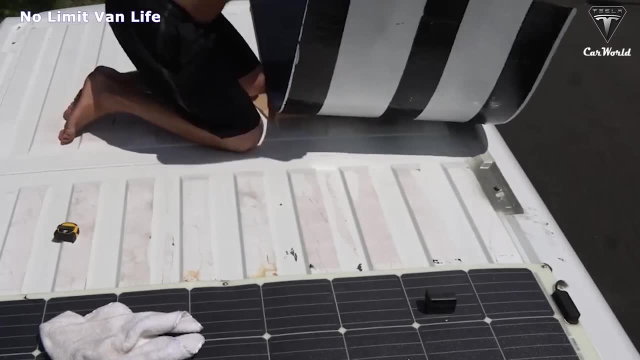 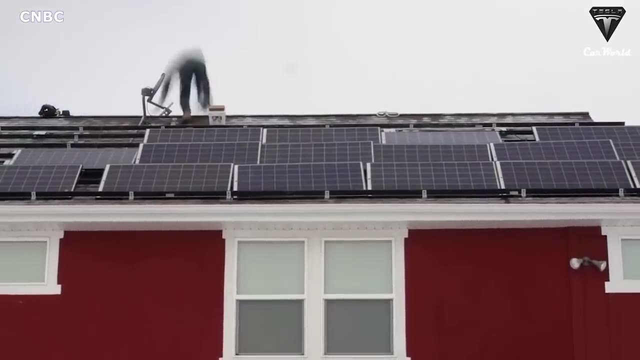 side of the junction in the absorber layer. Unlike silicon-based solar cells, these thin film solar cells are more stable, flexible, durable and easier to install And, as you know, traditional solar panels will become less efficient when it's overcast. This can be one. 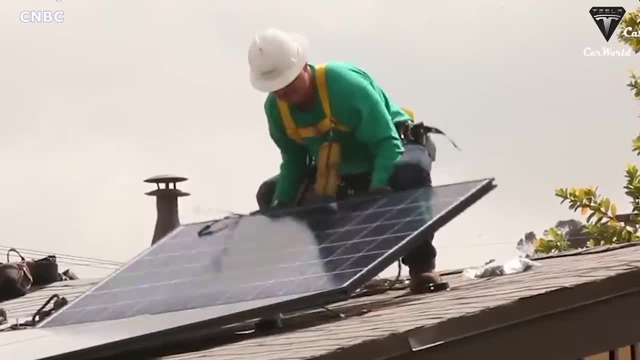 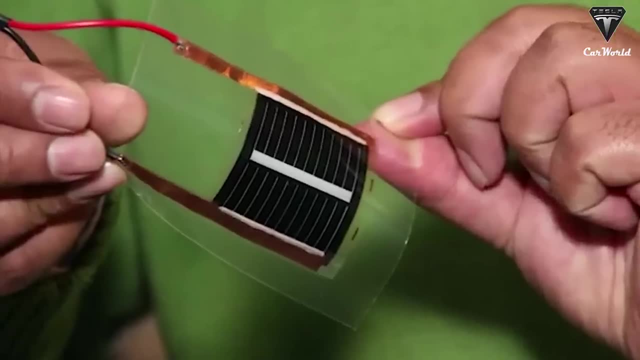 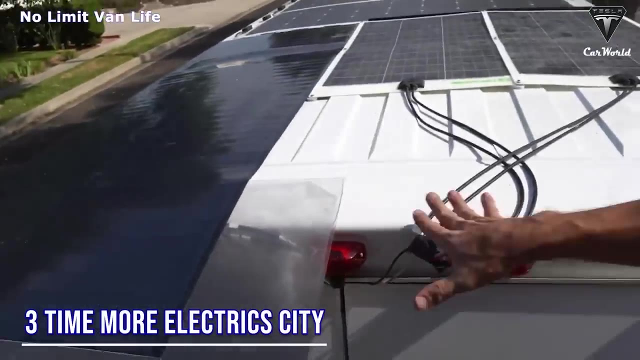 of the biggest setbacks for Tesla's solar panels, as well as other solar panels. But thanks to wire intensive copper-indium-gallium-selenide technology, Booge RV's flexible solar panel is more stable. It is said to be able to generate three times more electricity than your average. 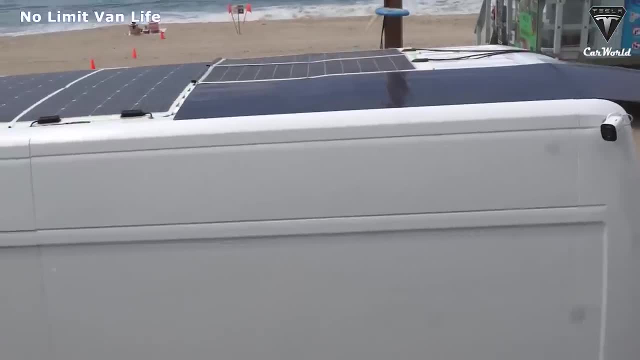 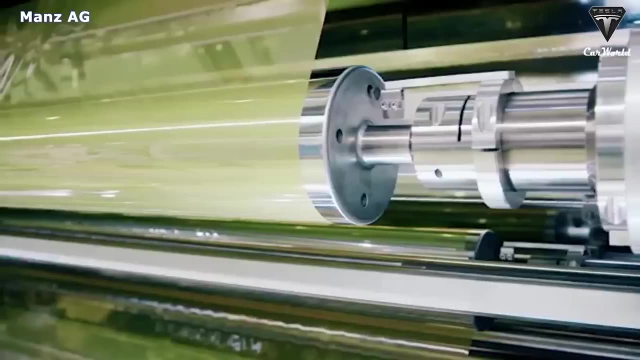 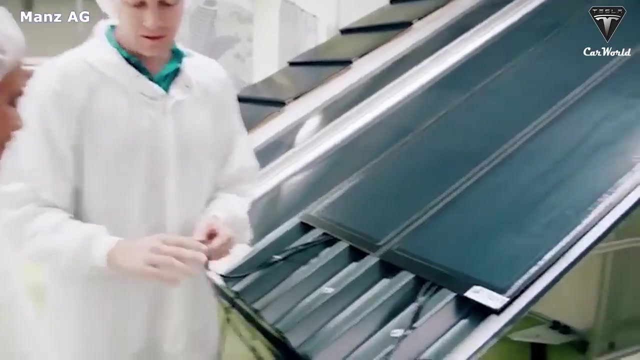 solar panel in low sunlight conditions. A flexible 200-watt 12-volt solar panel can produce 400 watts of power in the shade. Its modules deliver unprecedented efficiency. The cells within this solar panel are connected using a combination of series and parallel connections. This means that 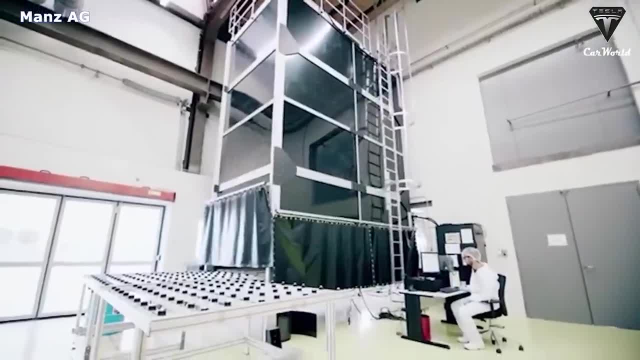 if you have a solar panel that is more stable than your average solar panel, you can generate more electricity. If one cell gets blocked by shade, it will still be able to produce power from any other areas left in the sun. In short, you might choose thin film solar panels to provide. 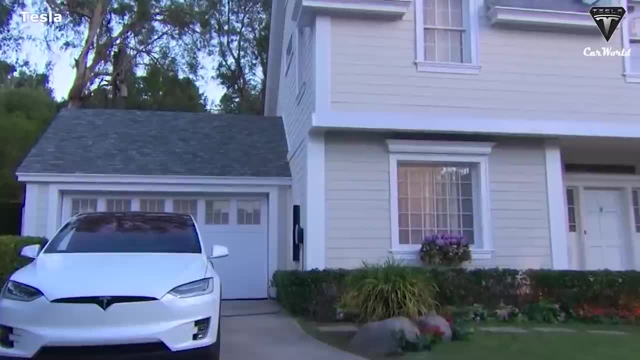 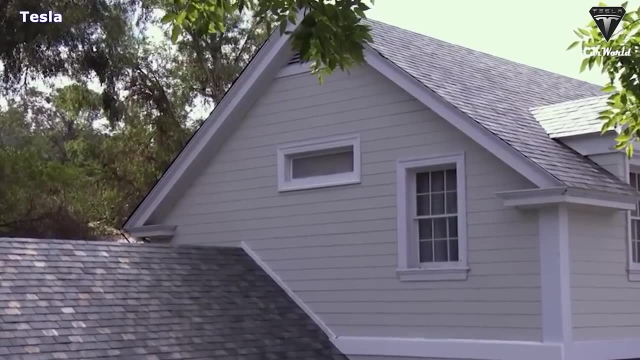 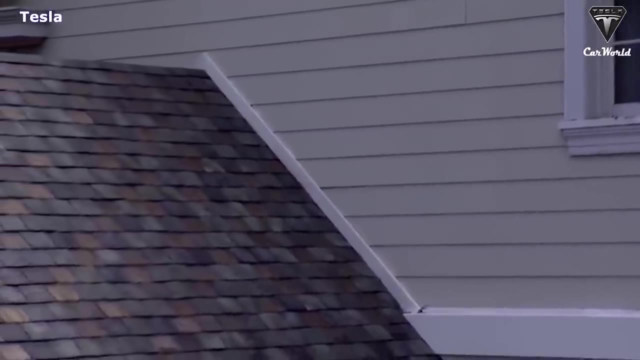 higher stability for your off-grid photovoltaic system. For comparison, a 200-watt Tesla solar panel produces 200 watts of energy per, but in reality it would produce about 70-80% of its rated power. This means that a 200-watt 12-volt solar panel would produce around 160 watts per. hour on a beautiful sunny day. If you have a solar panel that is more stable than your average solar panel, you can generate about 130 watts of energy per hour on a sunny day, But during an overcast, your Tesla solar panel will only generate about 130 watts of power output, which is not enough. 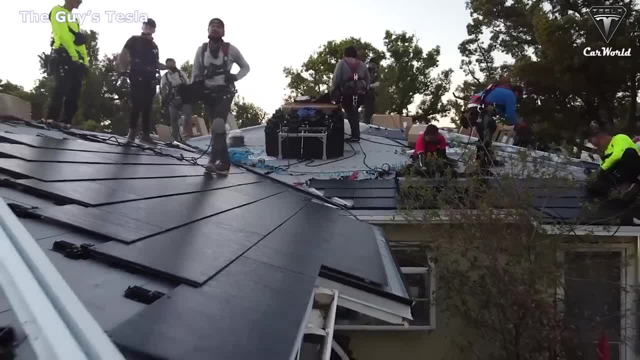 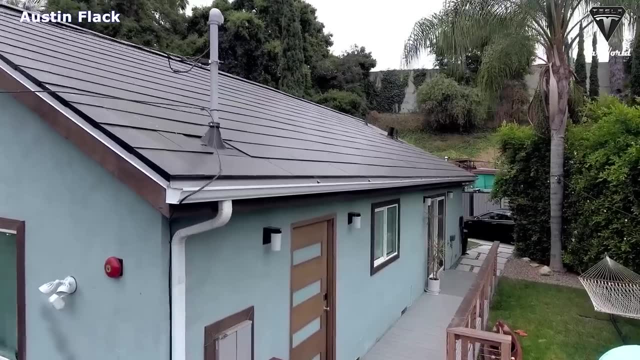 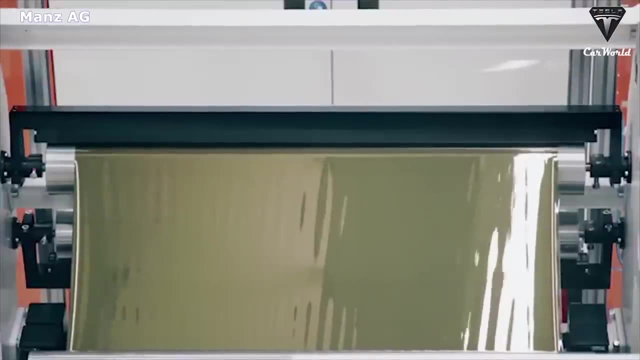 power for an entire house in Texas. The solar panels generating that power don't last forever. The Tesla solar panel lifespan is about 25-30 years, but luckily the lifespan is constantly improving as solar technology evolves globally. Bouge RV says the flexible solar panels can last. 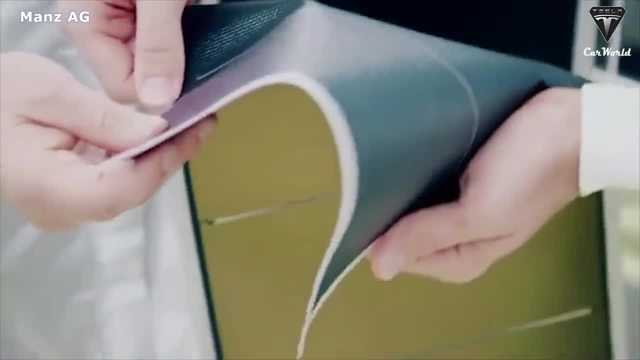 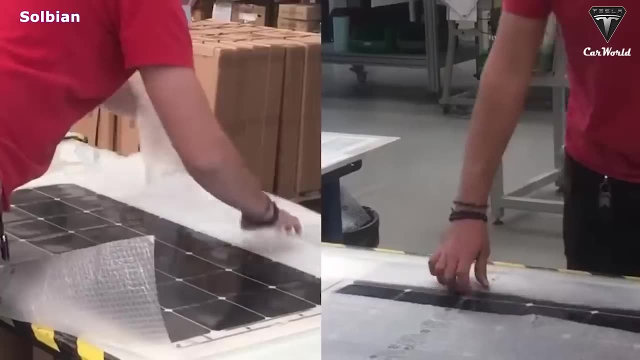 for 30 years when it has to work continuously, and can last up to 20 years. The solar panels can last up to 250 years if they are not in use. We can proudly say that Bouge RV's flexible solar panels are tough and rigorously tested. Bouge RV tests them through a high-pressure flushing test. 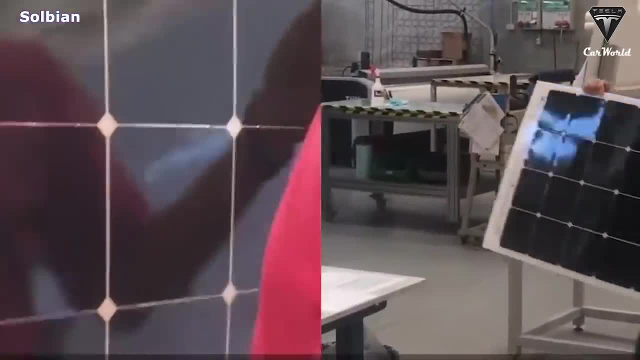 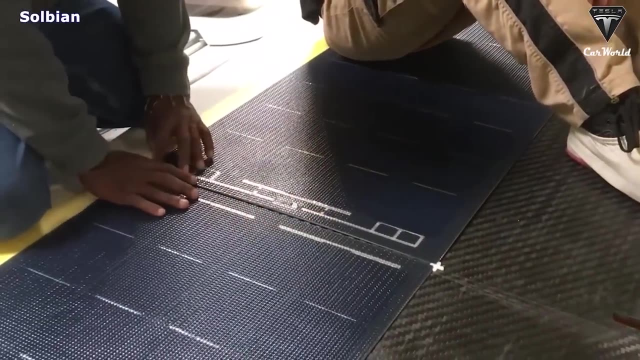 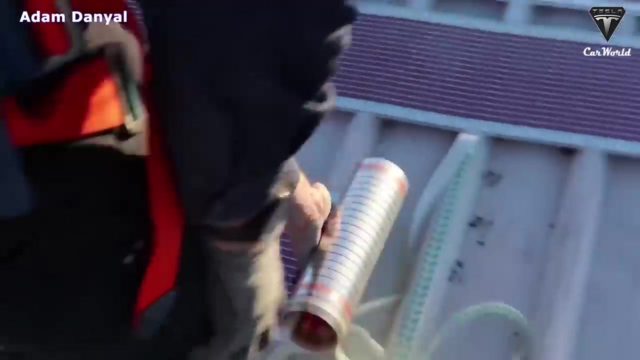 penetrating damage test and rolling limit test of automobile tires. Since this solar panel is designed for outdoor use on RVs and boats, it is also IP68 waterproof. This ETFE-coated flexible solar panel is waterproof and has improved rainfall drainage To lessen the influence of partial shade. Partial shade, This means you can slap it on the front. 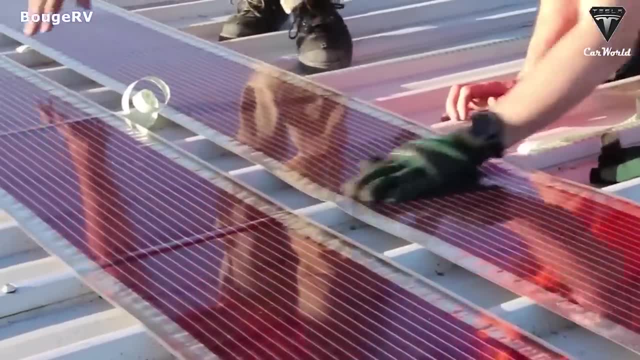 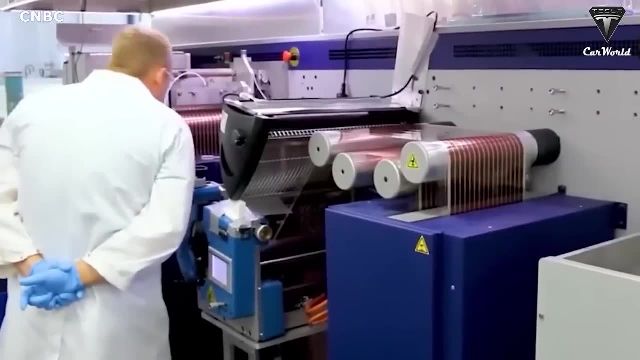 of your boat or have it outside your RV during a bit of rainfall, and you won't be risking any damage. The connectors and junction box are also IP68 waterproof, Therefore, it can operate well in a damp outdoor environment while outperforming a rigid panel. 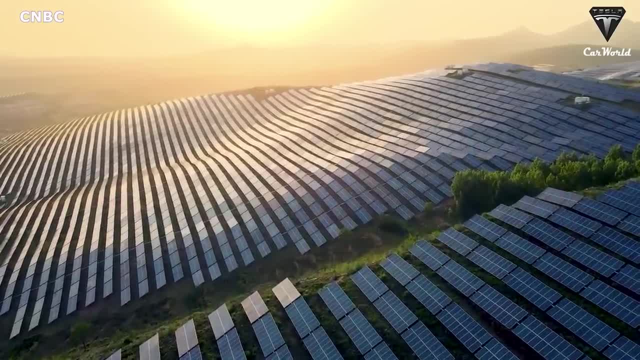 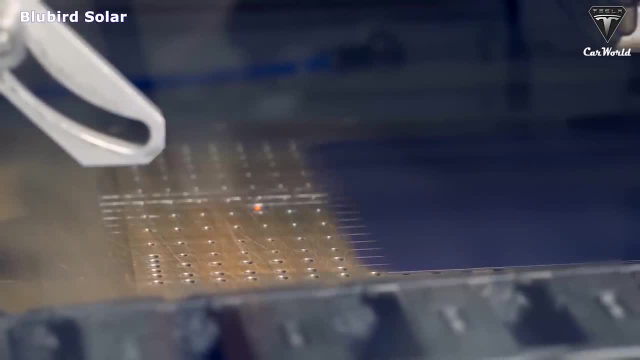 The weight of the 200-watt Tesla solar panel is 26.46 pounds, or 12 kilograms, while the new flexible solar panel only weighs 1.84 kilograms- only one-sixth of a rigid solar panel. Flexible panels are already. 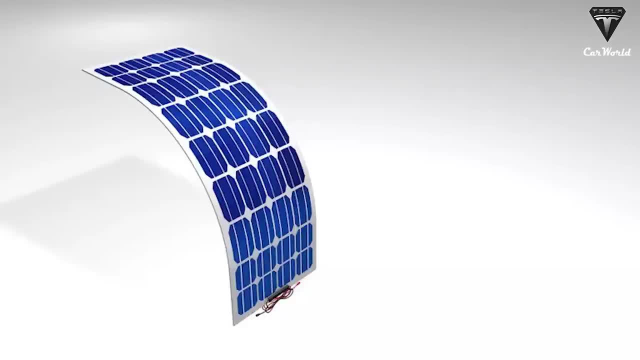 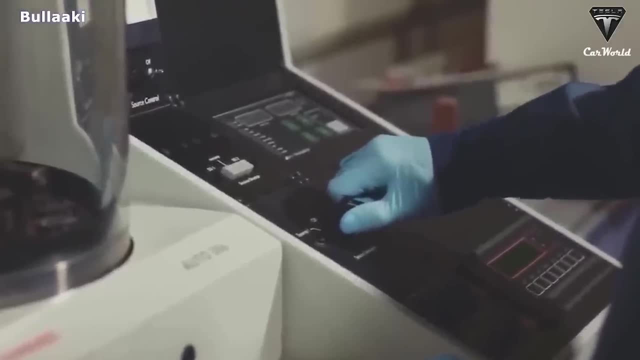 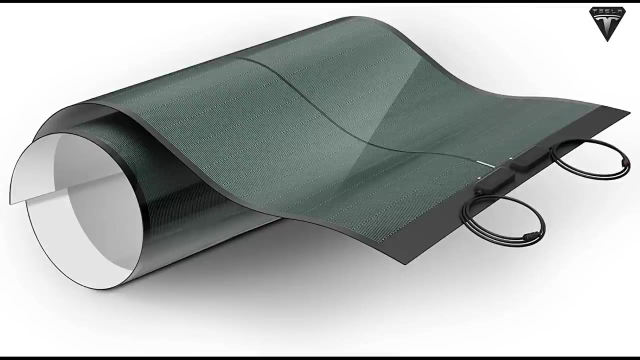 as the name suggests, more flexible than rigid panels and can be adapted to some surfaces, especially curved ones. The copper- indium- gallium selenide flexible solar panel is an upgrade of the ordinary flexible solar panel. If an ordinary flexible solar panel can be bent 150 degrees, 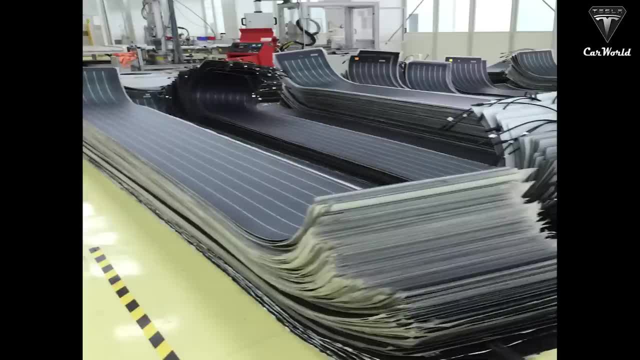 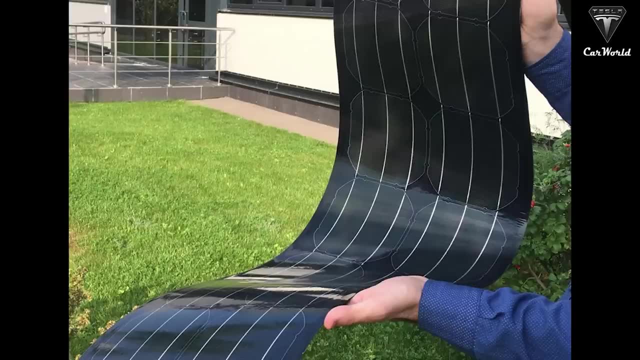 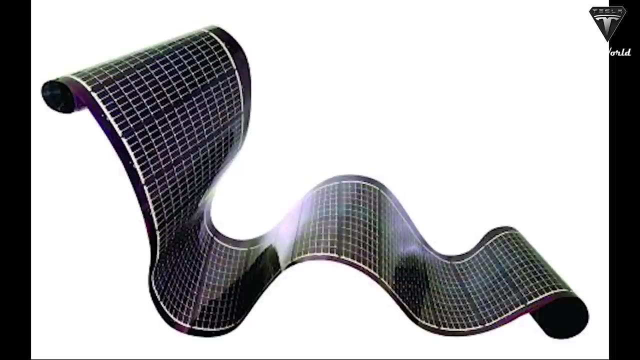 then this flexible solar panel can be bent to 360 degrees To achieve the real sense of bending. It can even be curved to a roll and adhere to any uneven surface and it's perfect to get a start in solar for your house And great for off-grid applications. 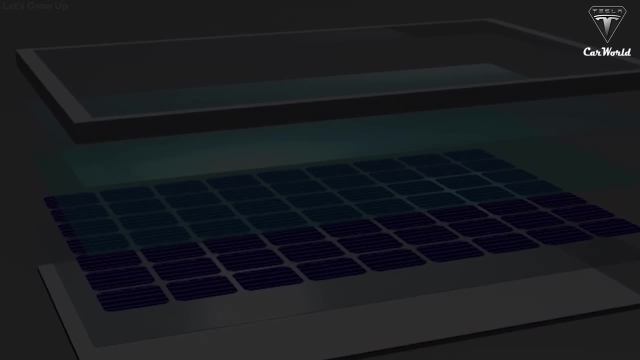 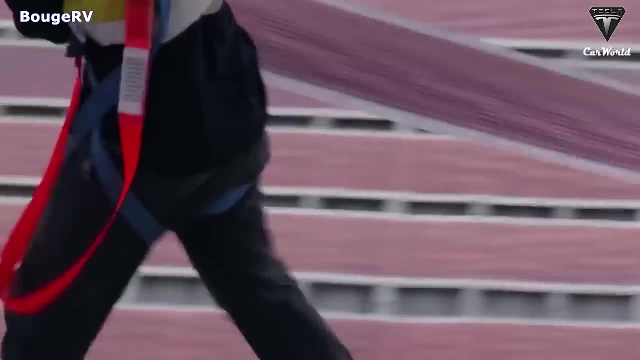 Use it for your RV, van, boat, truck and trailer. while on the road, The flexible panel provides you with the most stable efficiency per space If you're worried about your phone or any of your appliances running out of charge during a camping trip. 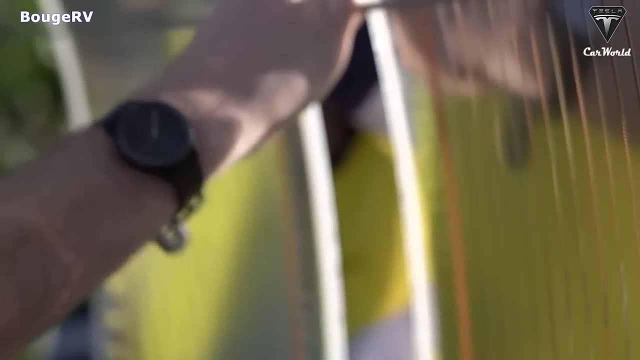 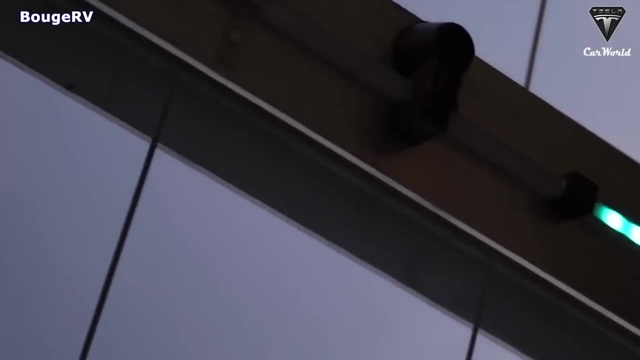 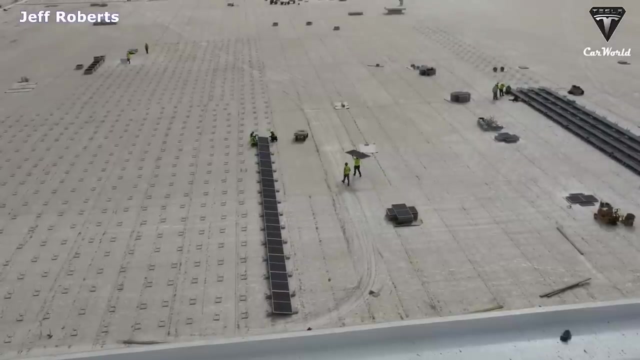 your car or long hike. a flexible solar panel can solve that problem. You'll need to attach the flexible solar panel to your backpack or tent and use the power it generates to charge your electronics. So what about the price of the new flexible solar panel, Tesla's solar panels, that? 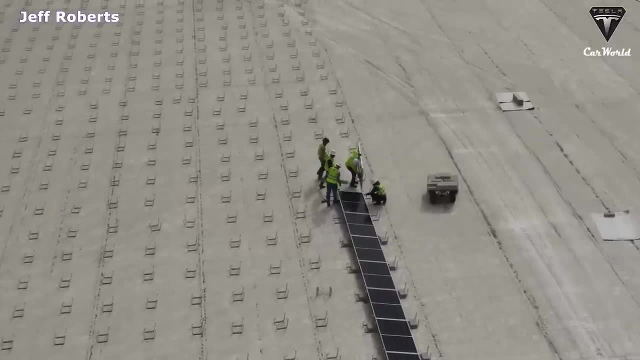 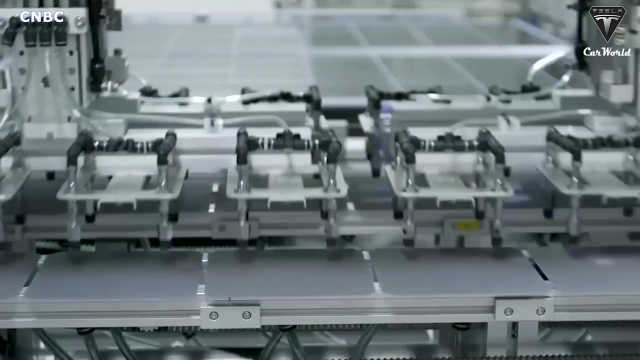 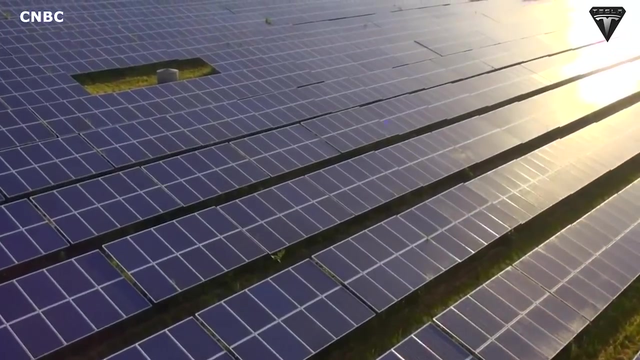 come in 100 or 200 watt, 12 volts with pre-drilled holes can cost at least $66.. On the other hand, with a deal from Buj RV, a 100 watt flexible solar panel for just $199.99 by using promo code AFF50.. This means you can. 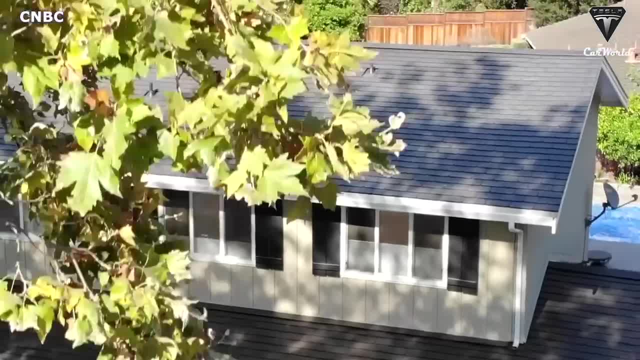 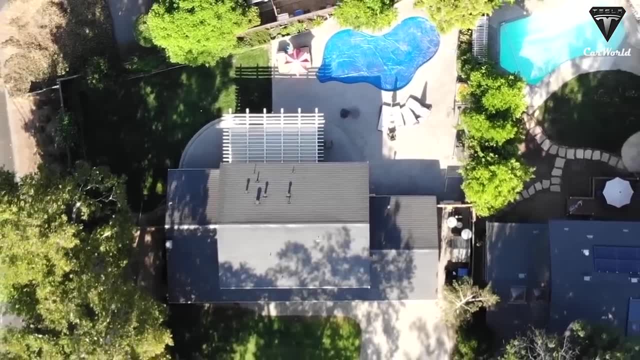 save $50.. It can be said that it is three times more expensive than Tesla's solar panels. But one thing you have to consider is, even though the price may be three times as expensive as the Tesla solar panel, it won't cost as much to install it. So you have to consider all the 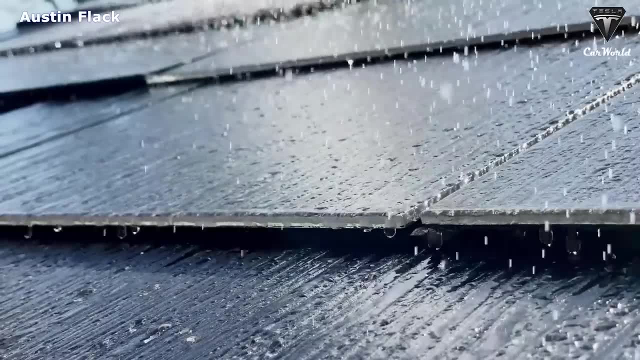 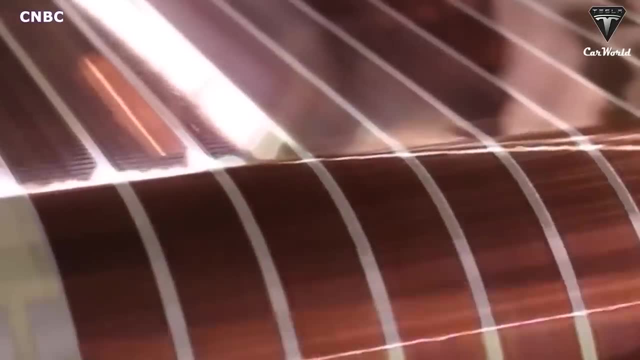 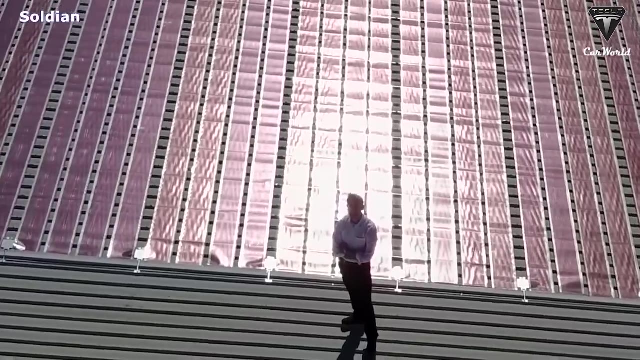 possible savings that you could get from installing flexible solar panels. Unlike some rigid solar panels that may require a professional to install, flexible panels are faster to install. Many flexible solar panels on the market come with adhesive backing and plug and play components, making it easier than ever to install your new solar system. The cost of labor for rigid panels: 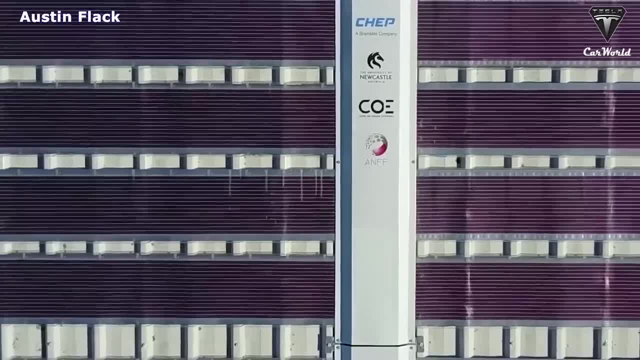 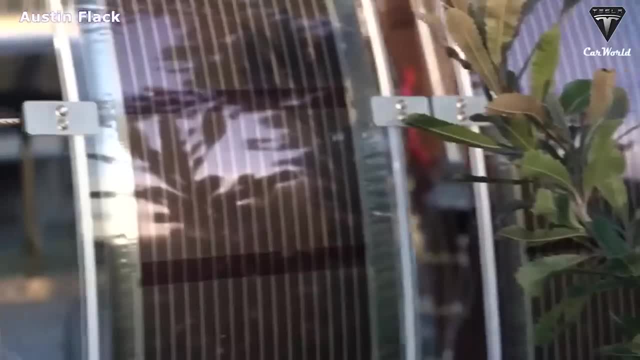 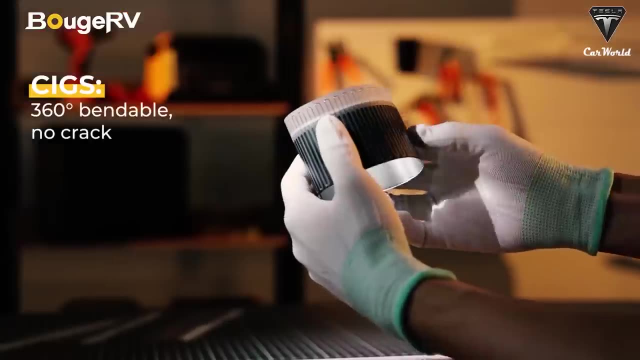 is expensive, whereas a flexible panel can be installed with only a tube of Sycaflex glue. Overall, copper, indium, gallium, selenide. flexible solar panel technology requires fewer materials and less energy to produce. If you're an outdoor enthusiast, then a flexible solar panel is a 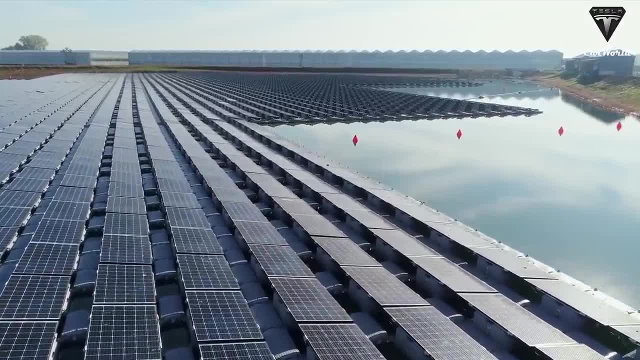 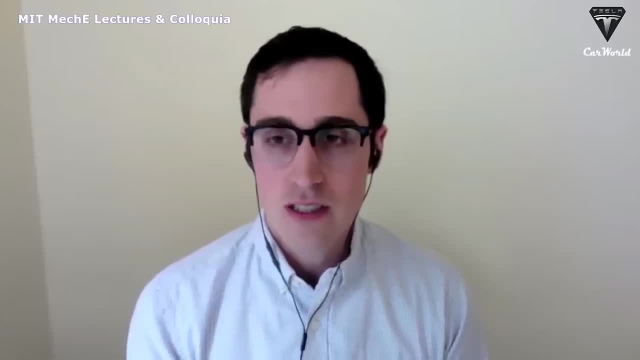 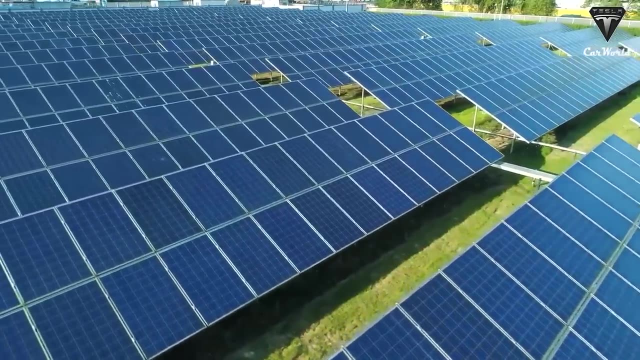 game changer. Maybe in the future, this technology will also have the potential of reducing costs and become a cheaper solar alternative. in the Lone Star State, You can access production at larger scales, which is one of the bottlenecks to entry into an application space like energy storage, where you need to deliver. very large systems. I think that would be probably the most exciting first application for TPVs. One new solution by researchers at MIT called thermophotovoltaics will blow your mind. What breakthrough advantages will it have and can it provide the energy storage solution we've been? 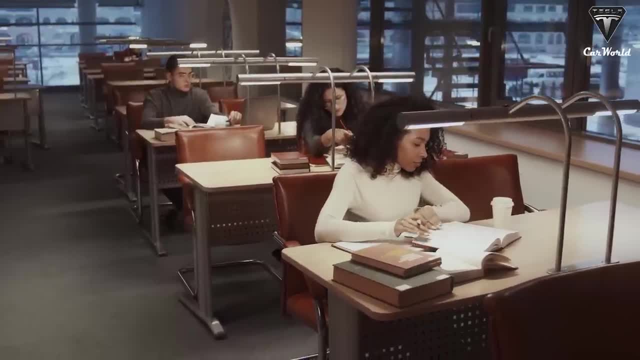 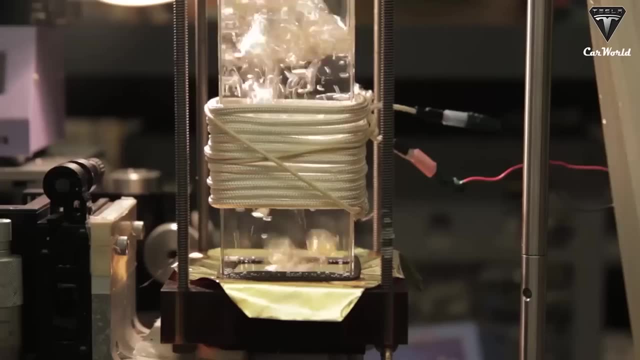 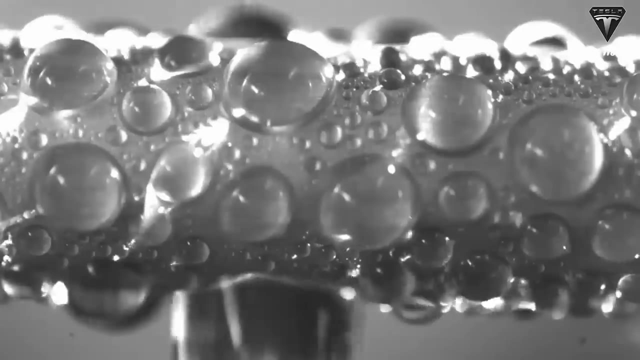 looking for. More than 90% of the world's electricity comes from sources of heat such as coal, natural gas, nuclear energy and concentrated solar energy. For a century, steam turbines have been the industry standard for converting such heat sources into electricity. On average steam. 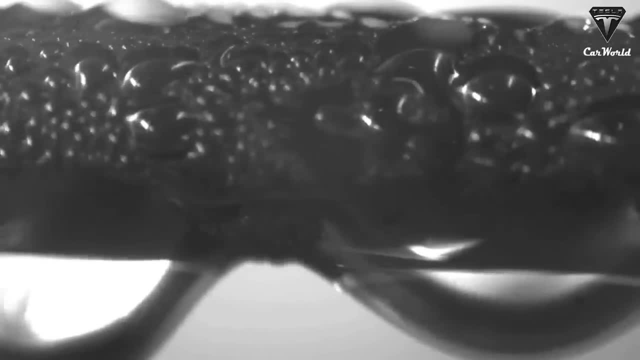 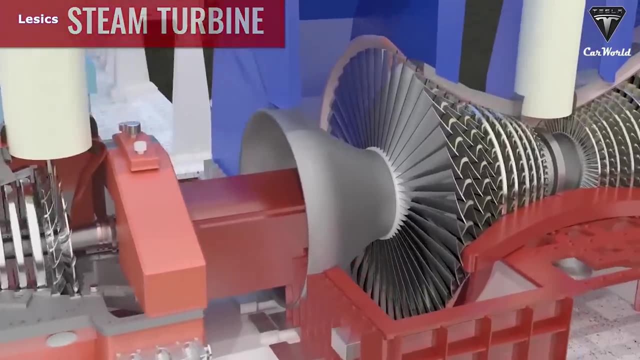 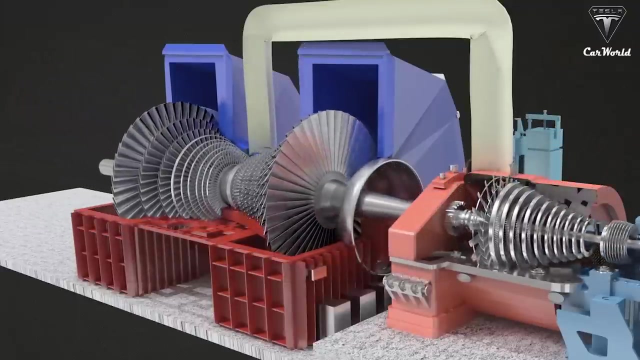 turbines reliably convert about 35% of a heat source into electricity, with about 60% representing the highest efficiency of any heat engine to date, But the machinery depends on moving parts that are temperature limited. Heat sources higher than 2,000 degrees Celsius would be too hot for turbines. 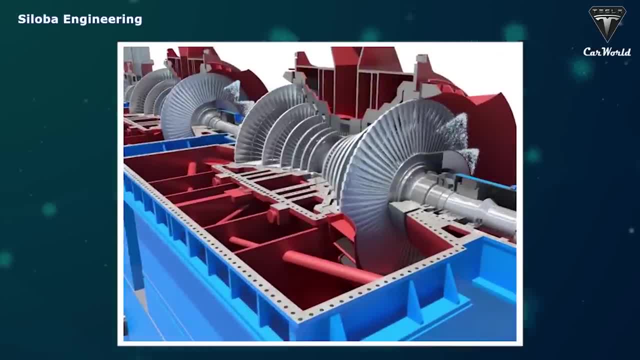 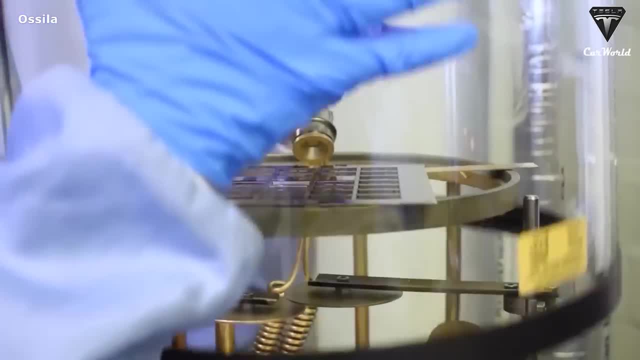 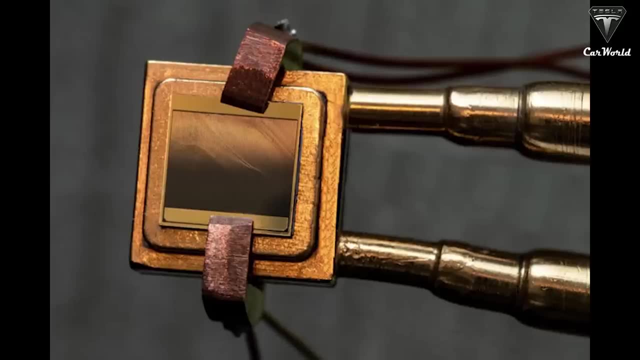 In recent years, scientists have looked into solid-state alternatives that could potentially work efficiently at higher temperatures. Engineers at MIT or Massachusetts Institute of Technology and the National Renewable Energy Laboratory, or the NREL, have designed a heat engine with no moving parts. Their new demonstrations show that it converts heat to electricity with over 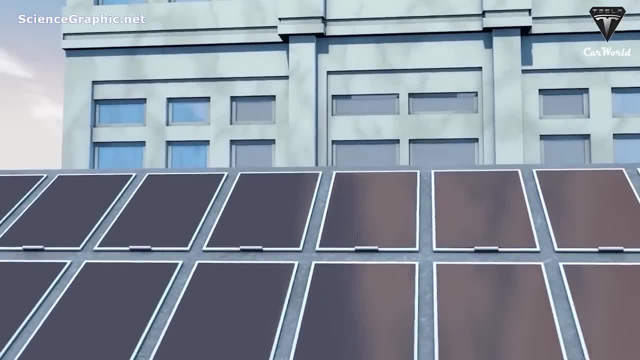 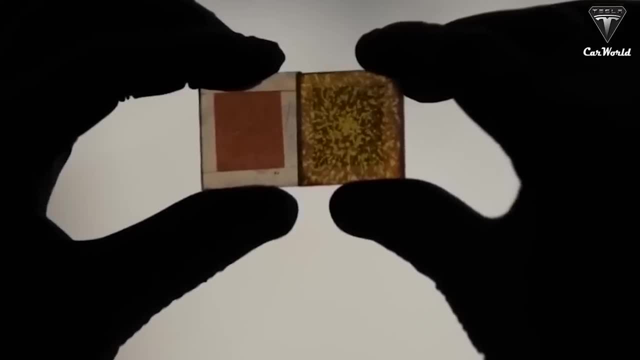 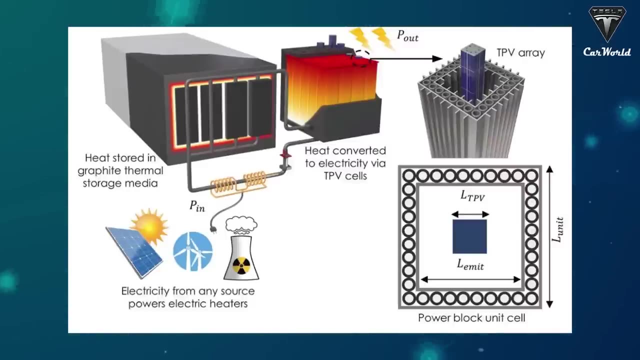 40% efficiency. It's a very competitive level of performance compared to the most efficient type of energy available today, which is nuclear power, And the heat engine is thermophotovoltaic or TPV cell, similar to a solar panel's photovoltaic cells that passively capture high-energy photons from. 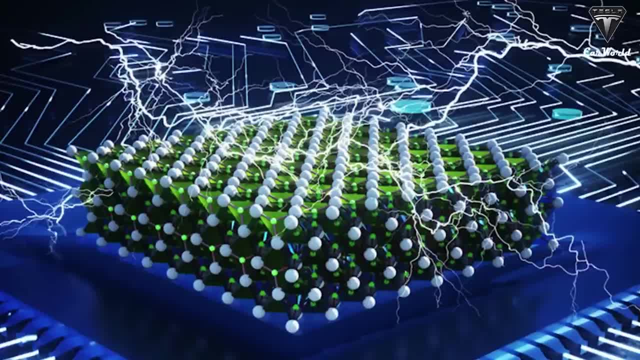 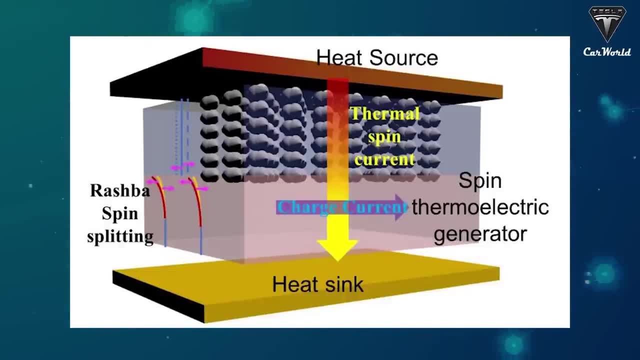 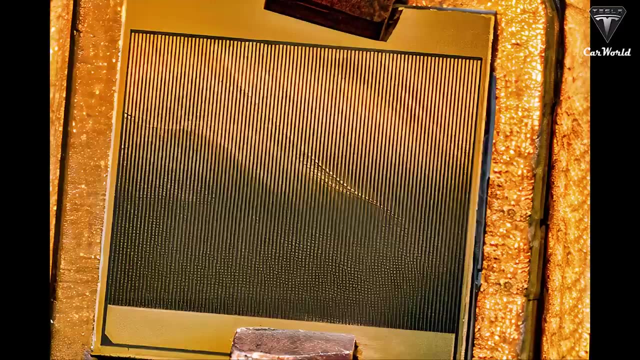 a white-hot heat source and converts them into electricity. The cell is fabricated from three main regions – a high bandgap alloy, which sits over a slightly lower bandgap alloy, and underneath, which is a mirror-like layer of gold. The first layer captures a heat source's highest energy photons and converts them into. 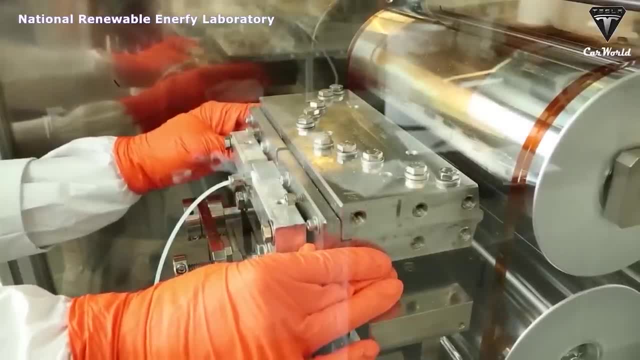 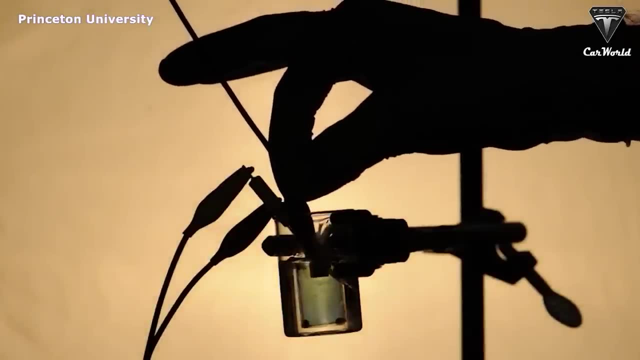 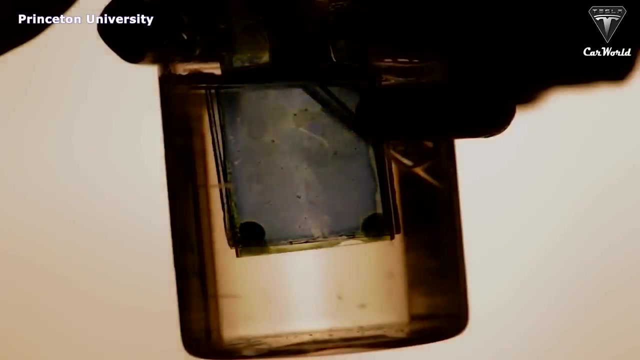 electricity, while lower energy photons that pass through the first layer are captured by the second and converted to add to the generated voltage. Any photons that pass through this second layer are then reflected by the mirror back to the heat source rather than being absorbed as wasted heat. 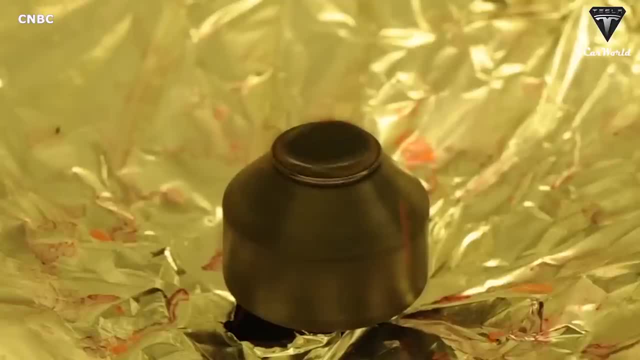 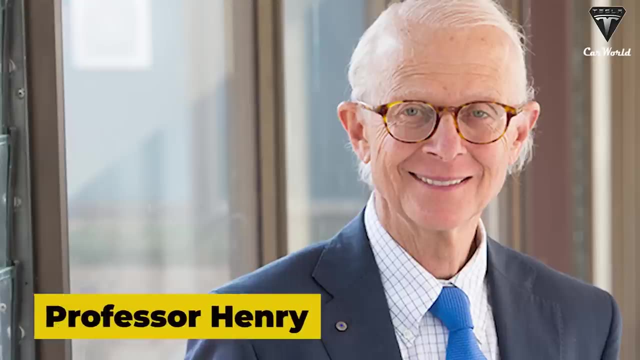 The team's design can generate electricity from a heat source of between 1,900 to 2,400 degrees Celsius, or up to about 4,300 degrees Fahrenheit. According to Professor Henry, the rate at which heat leaks out of the blocks is proportional. 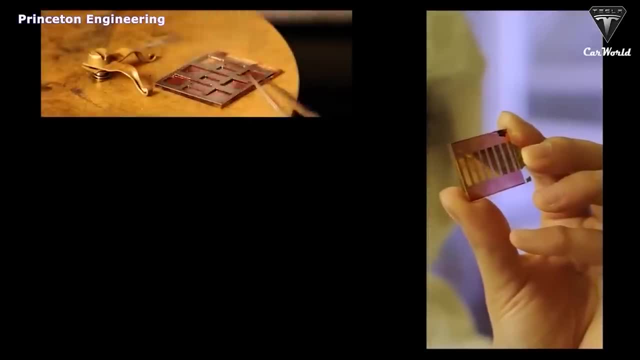 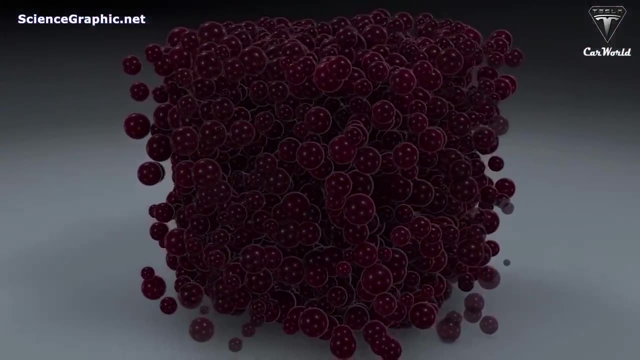 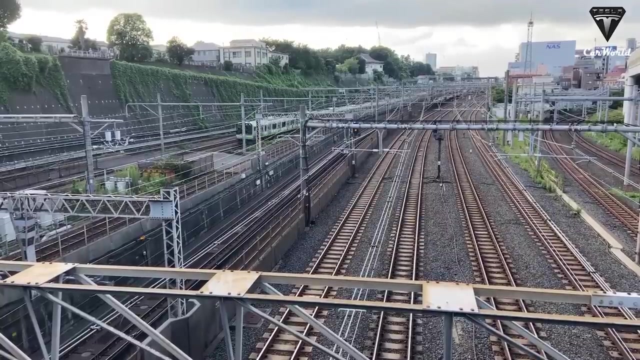 to their surface area, whereas the amount of energy they can store relates to their volume. They will take months to cool down, making them the perfect medium for storing thermal energy. The average battery energy storage capital costs in 2019 was at $589 per kilowatt hour. 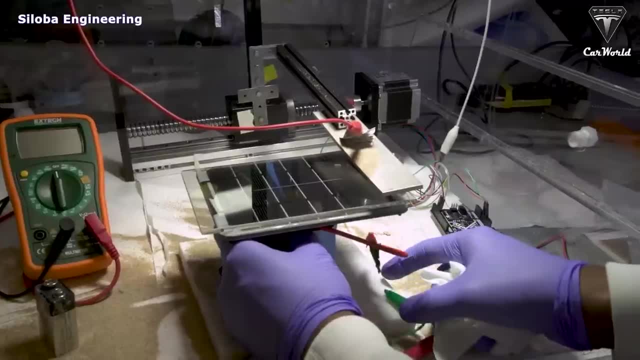 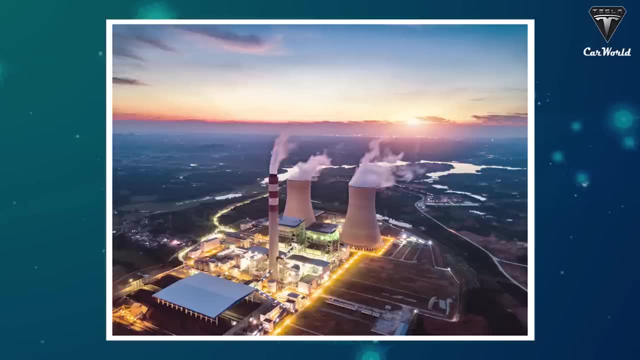 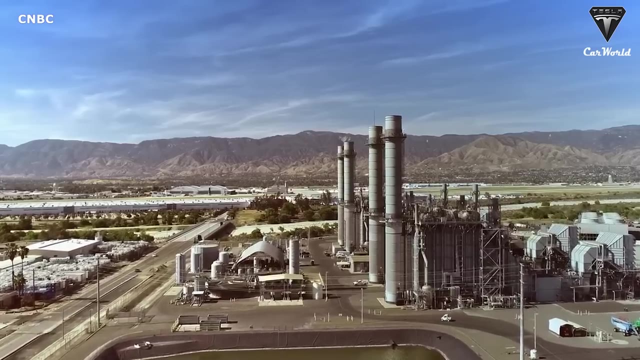 After considerable research, Henry and his team estimate that this system could store energy at a fraction of the cost, at around $10 per kilowatt hour of capacity, while nuclear power is 1,300 times more expensive. Capital costs for nuclear power plants range between $7,800 to $12,800 US dollars per kilowatt. 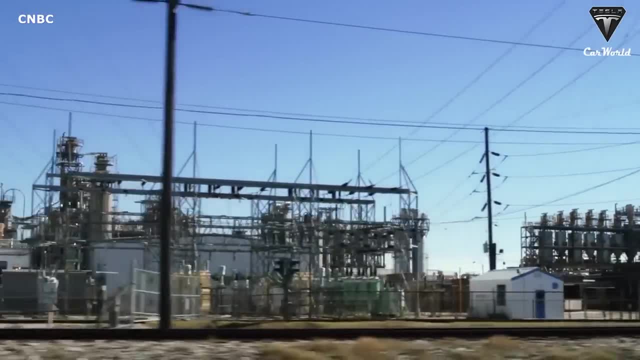 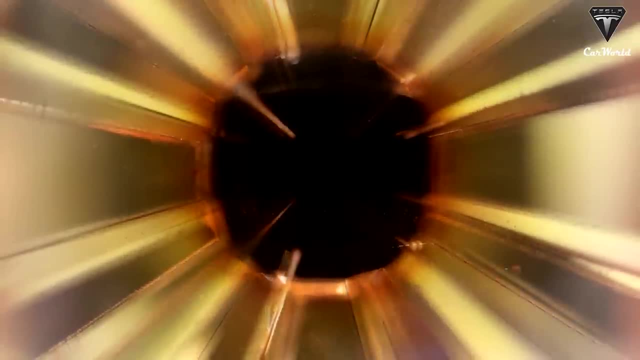 Does the cheaper price make up for the lower efficiency? Well, let's talk a little bit about how much power that would make. These cells could reach that 40% efficiency mark, so a one-square-meter cell could generate around 100 kilowatts. 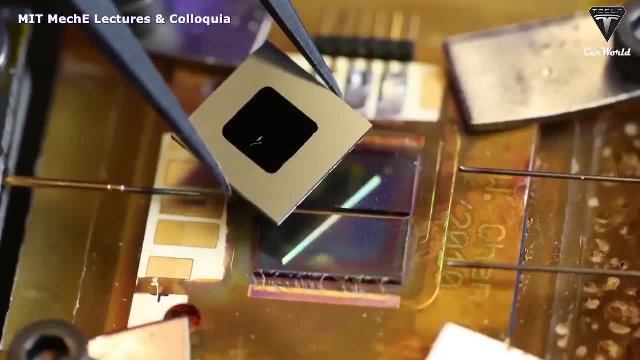 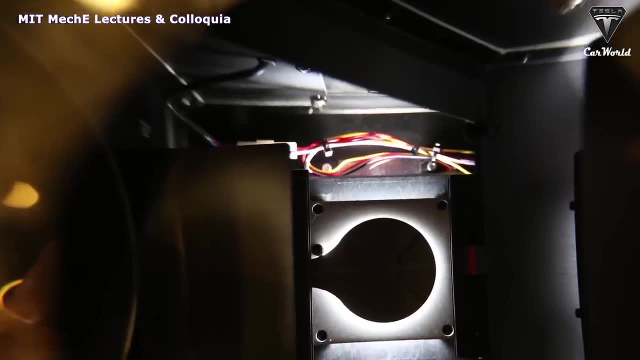 For comparison, the power per area of nuclear power facilities is also about 100 kilowatts per square meter. So an array of 30 by 30 modules, about 900 square feet, will have a total capacity of around 90,000 kilowatts or close to 100 kilowatts. 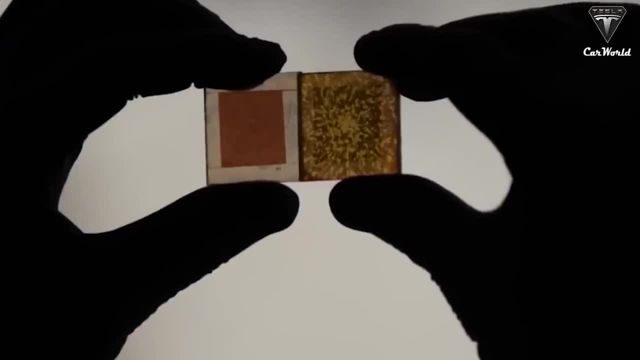 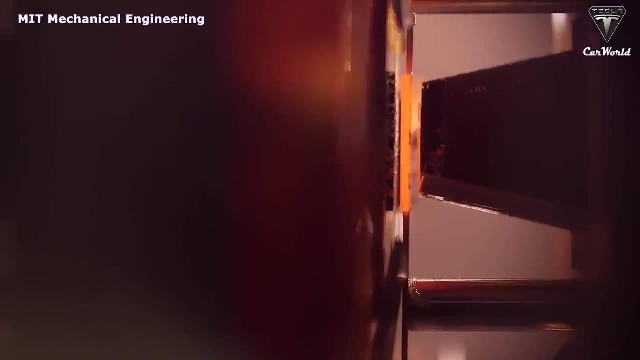 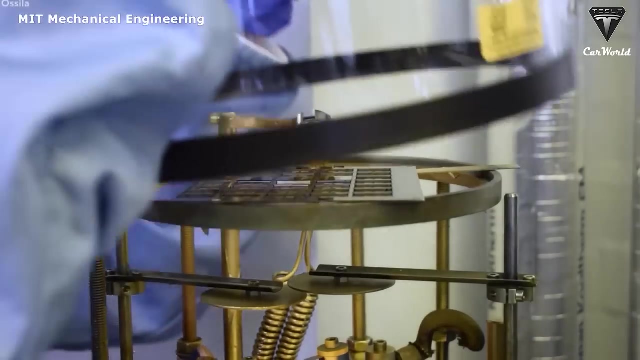 That's a lot. The graphite blocks can hold enough heat to keep the cells generating power for roughly 10 hours. 100 megawatts per hour for 10 hours means it could provide 1,000 megawatt hours or 1 gigawatt- enough to power tens of thousands of homes. 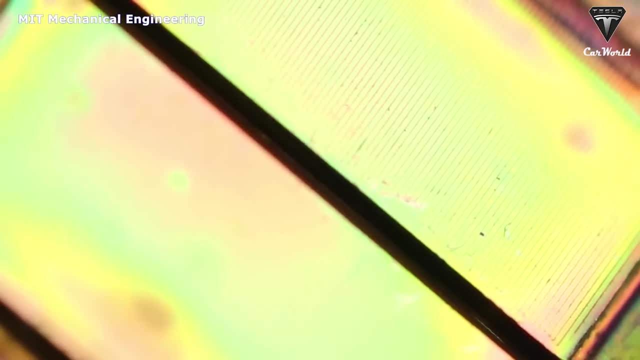 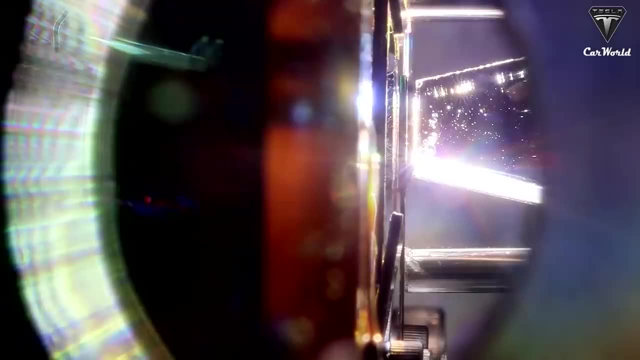 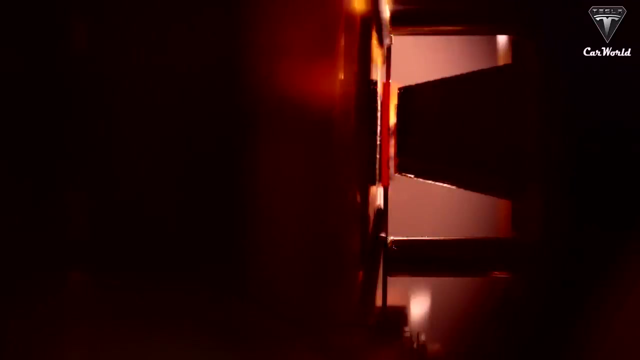 Moreover, TPV cells can deliver energy instantly, the same way traditional solar cells would. This would make them ideal for grid-scale applications. 3. In a grid-scale thermal battery, the system would absorb excess energy from renewable sources like the sun and store it in heavily insulated banks of hot graphite. 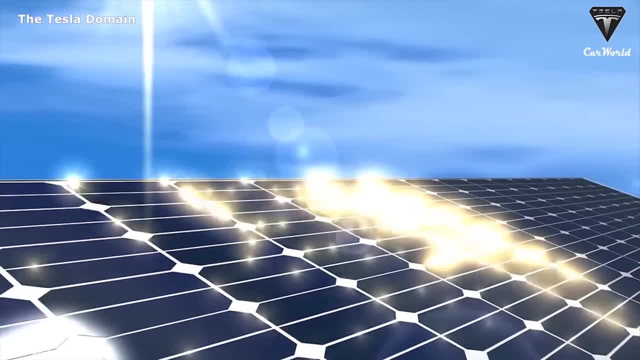 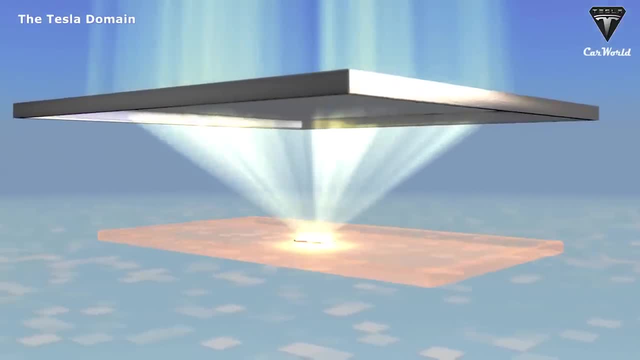 When needed. the TPV cells could then convert that heat to electricity and send it to the power grid. The experimental cell was just a square centimeter, so the team would have to ramp that up to about 10,000 square feet for grid-level power. 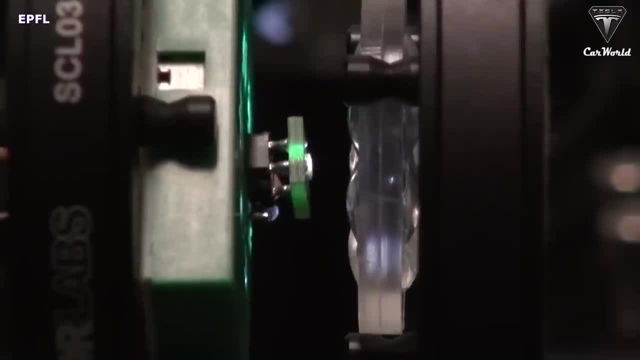 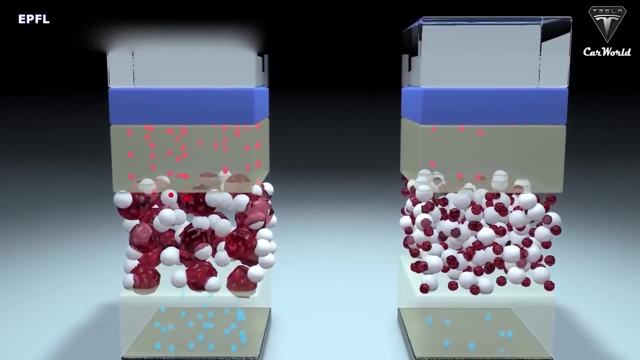 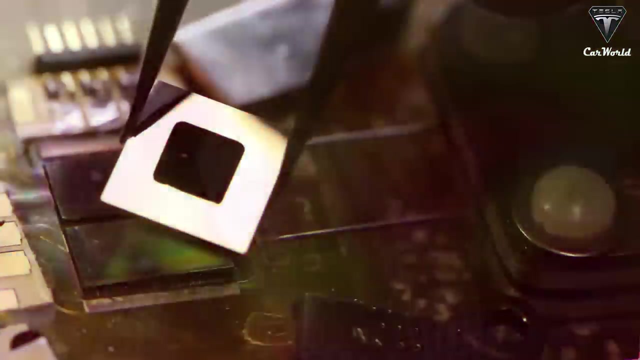 4. A nuclear energy facility has a small area footprint, requiring about 1.3 square miles per 1,000 megawatts of installed capacity. TPVs take little space to implement but they are as efficient as nuclear power. As of right now, a company plans to roll out a 1-megawatt-hour pilot system by the end. 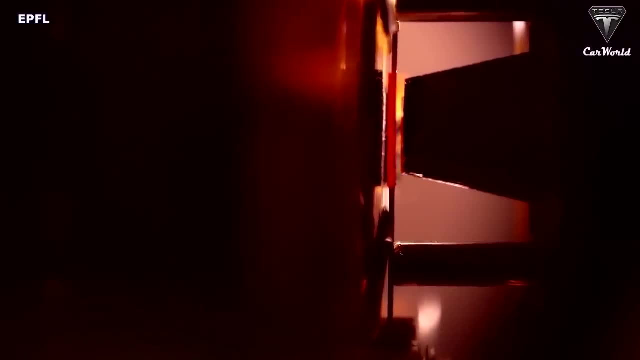 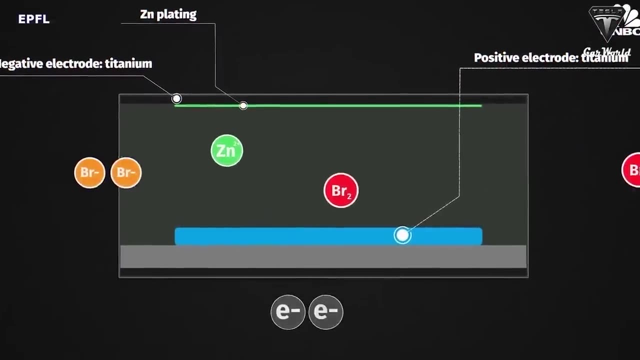 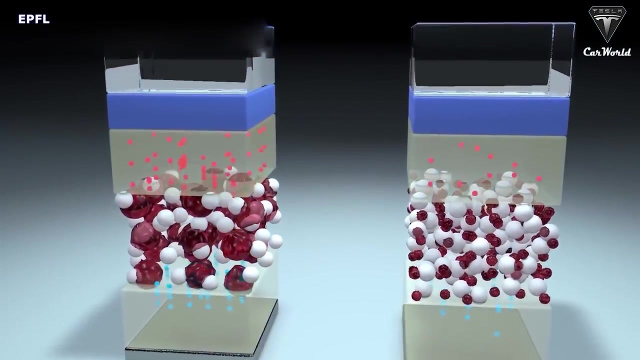 of 2022, with plans to eventually implement a 50-megawatt-hour commercial scale system by 2026.. 5. They also hope to further improve the cell's efficiency to 50 percent by increasing the fraction of unusable radiation they reflect by 97 to 98 percent. 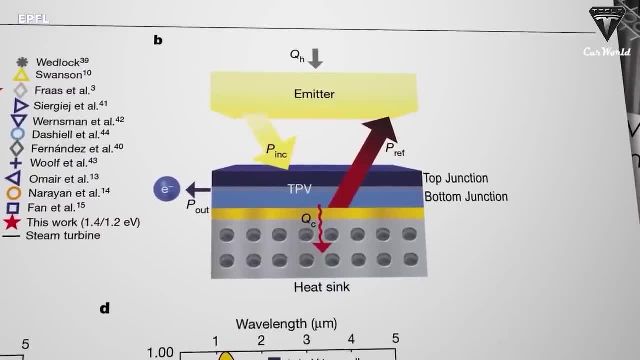 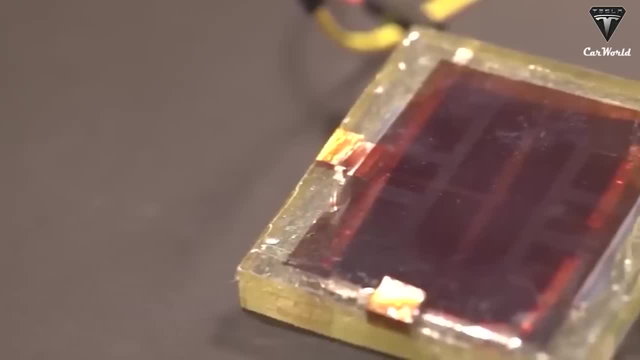 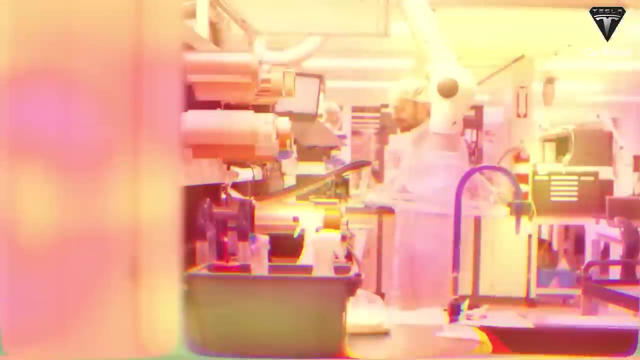 Thus, we could start seeing TPV systems co-located at power plants or smelters to improve efficiency and absorb some of that lost heat. Indeed, the opportunities abound, but before we get ahead of ourselves, we need to see how this pilot plant performs. 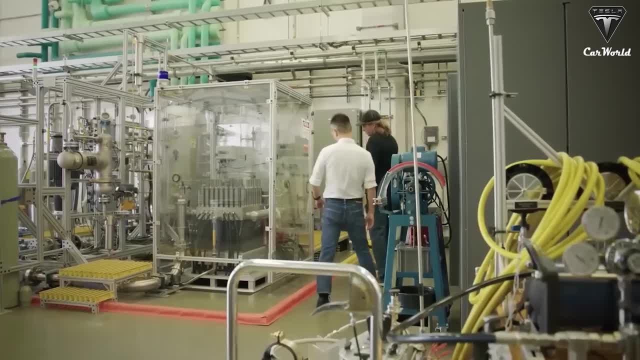 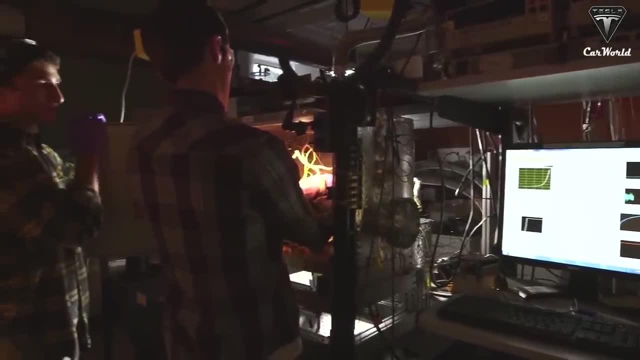 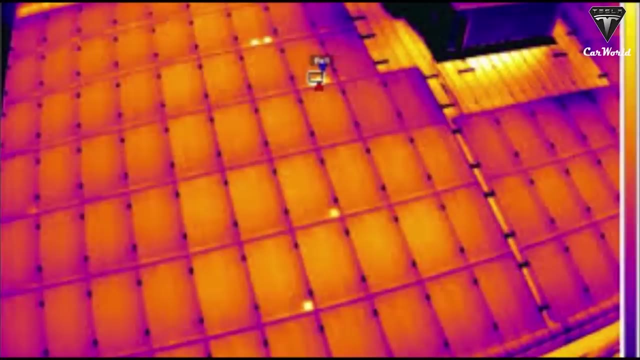 6. It's not super promising, but there are still lots of challenges that TPV needs to solve. 7. Moving heat requires very advanced, complex pumps and systems to cope with all that heat. Moreover, the system is very expensive to invest in and is still under development in. 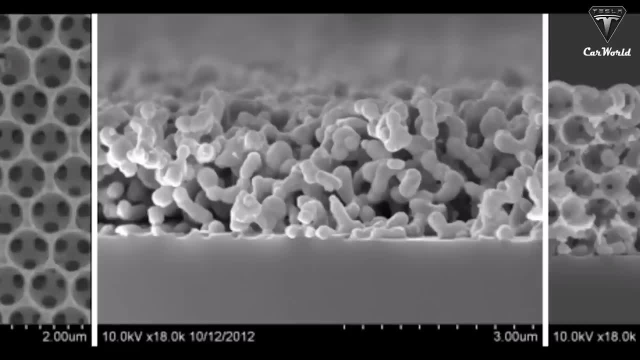 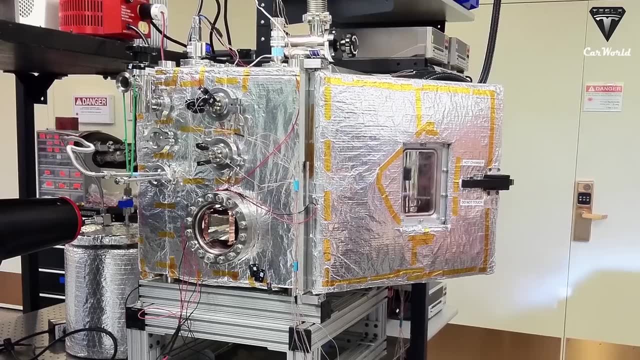 the lab Plus. blasting TPV cells with such intense heat and light is another new challenge engineers haven't faced before. The main problem with molten tin is that if something goes wrong and they don't get hot enough and the heat drops below the melting point, all of the tin solidifies, so the 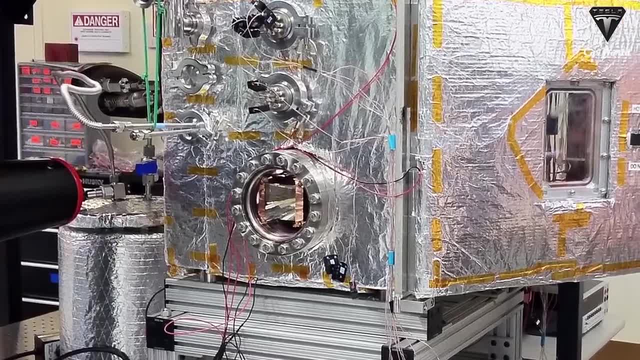 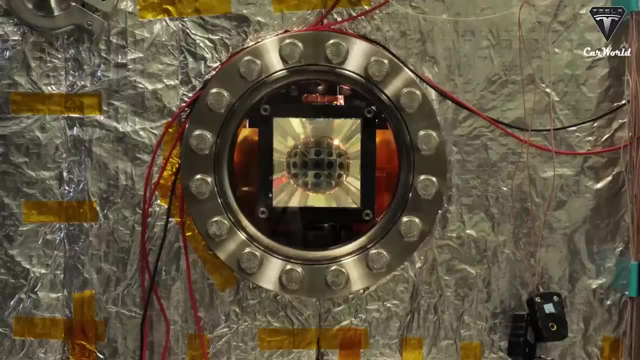 system cannot ever be allowed to cool down, even with sufficient cooling to keep the panels from overheating. 8. When it comes to nuclear power, uranium extraction, transporting and processing all produce emissions. The long and complex construction process of nuclear power plants also releases CO2,. 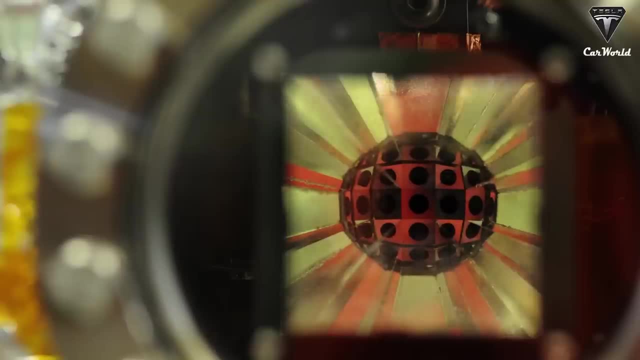 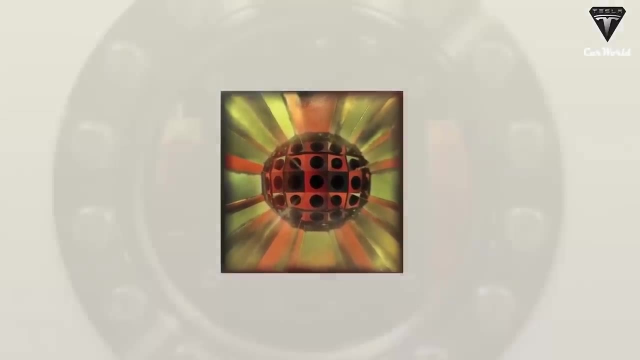 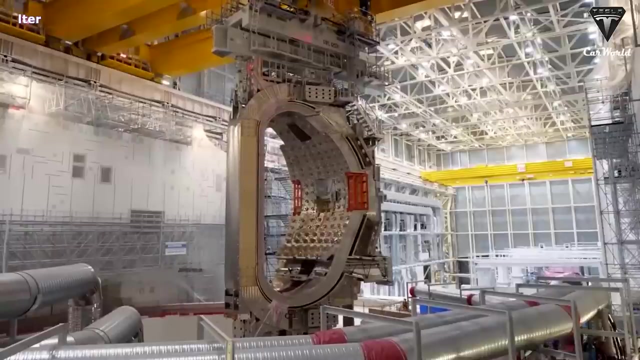 or carbon dioxide, as does the demolition of decommissioned sites. Moreover, if a nuclear power plant accident occurs, or otherwise known as a meltdown, the environment and surrounding people could be exposed to high levels of radiation. The 2011 accident at the nuclear power plant in Fukushima, Japan, is one of the worst nuclear 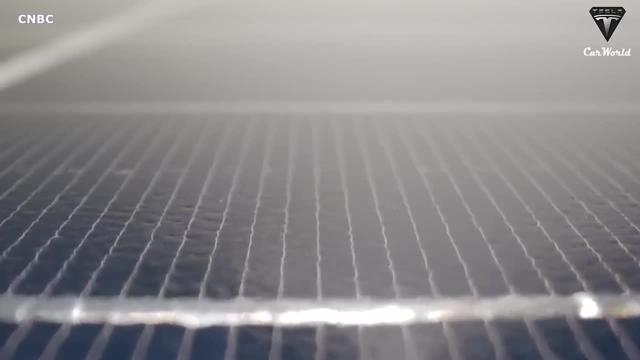 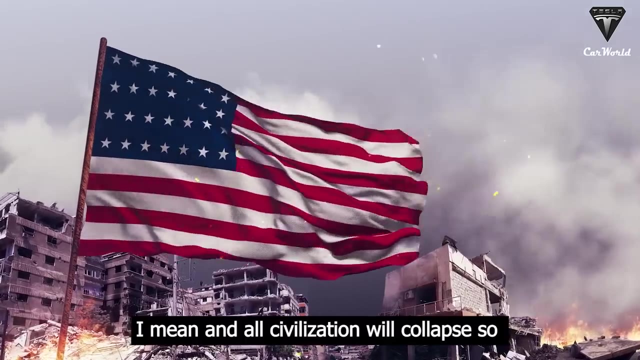 disasters in history. The reactors were destroyed by a tsunami following a major earthquake. 9. We will eventually run out of energy and die. 10. Civilization will collapse. 11., 12. There are no ways to produce energy in a renewable manner. 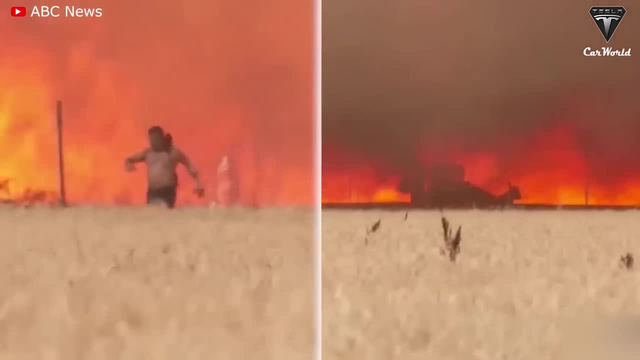 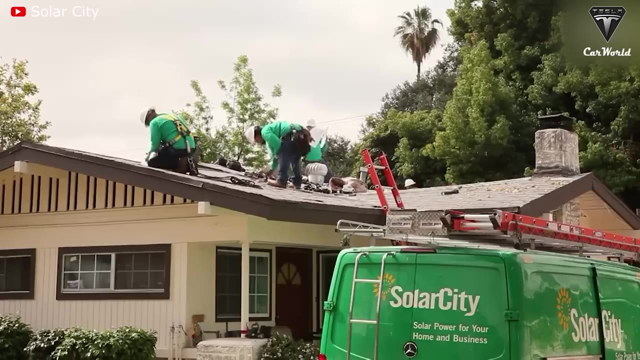 Texans have been suffering from a brutal heat wave for the last six weeks, and every morning they worry about the condition of the state's electricity grid. So Elon Musk has developed a low-cost renewable energy source that may end the Texas emergency. What energy source could he be talking about? Tesla announced that its solar deployments had increased by 25% year-over-year in the second quarter to 106 megawatts Energy generation and storage revenue. This amounted to $866 million, which is equivalent to around 5.1% of Tesla's total revenue in. 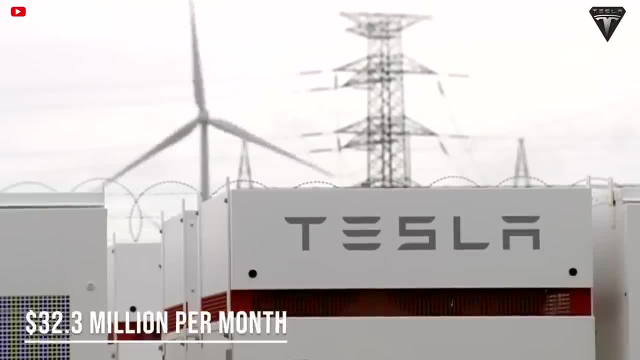 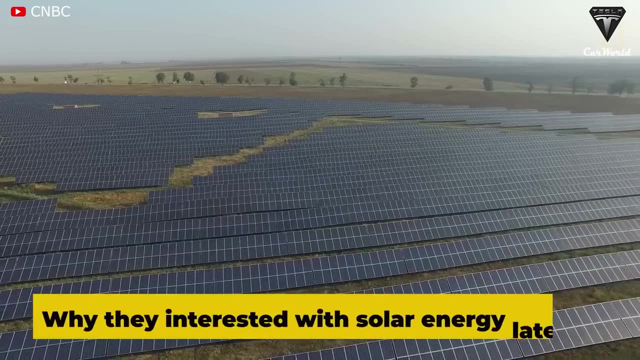 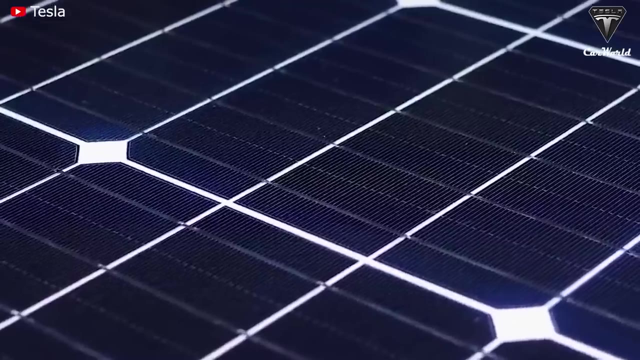 the quarter, with gross profit from the division standing at $32.3 million per month. This is Tesla's strongest quarterly result in over four years. so why is there so much interest in solar energy? lately, In an interview, Elon Musk introduced a cheap solar power system specially tailored for 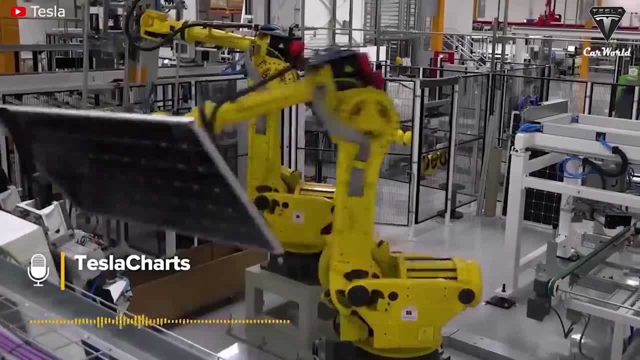 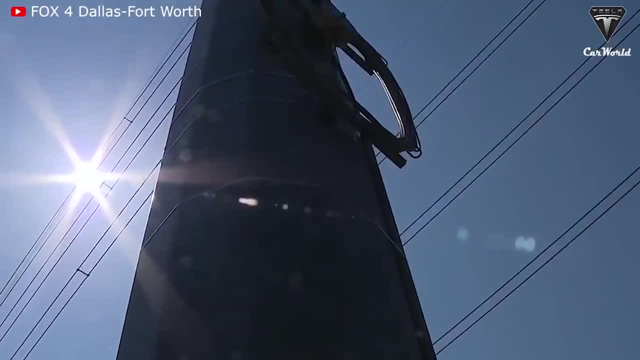 Texas, And we're going to show you 10.. The electricity from this new system is already cheaper than grid electricity costs. Having spoken with a Texas resident, the grid cost in March of 2022 was $0.15 per kilowatt. hour, a rise of 22.81% year-over-year For the Tesla's solar panels. his cost is fixed at $108.63 per month, which is the financing cost of the panels. We can see that the solar costs are higher in the winter and lower in the summer because 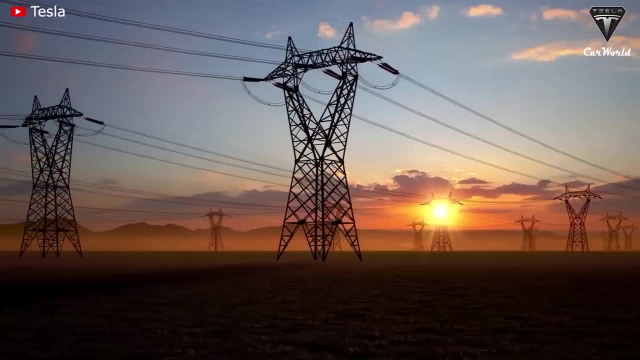 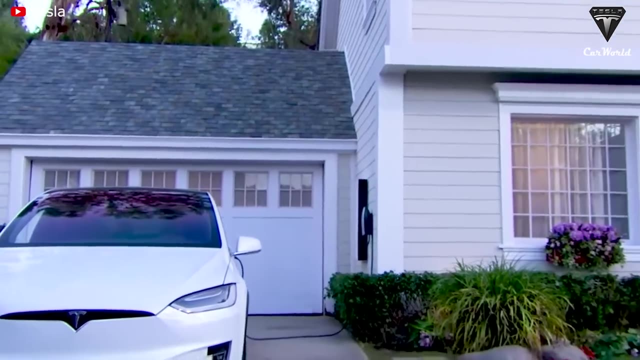 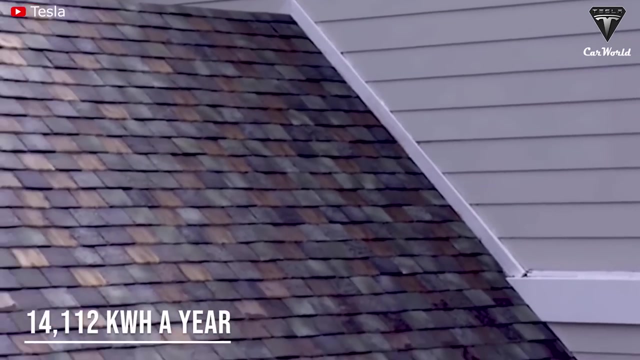 there is less sun available During the summer, his solar cost drops down to $0.07 per kilowatt hour. Ignoring installation costs, the average home in Texas uses 1,176 kilowatt hours a month, or 14,112 kilowatt hours a year. A large Tesla solar system of 11.34 kilowatts can produce an average of 43 to 58 kilowatt hours per day, equivalent to 1,500 kilowatt hours per week. That's a lot of solar energy. 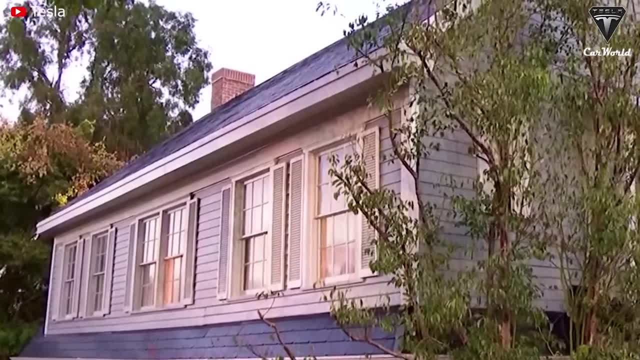 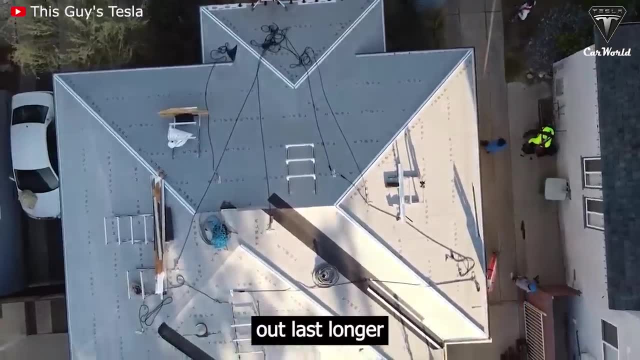 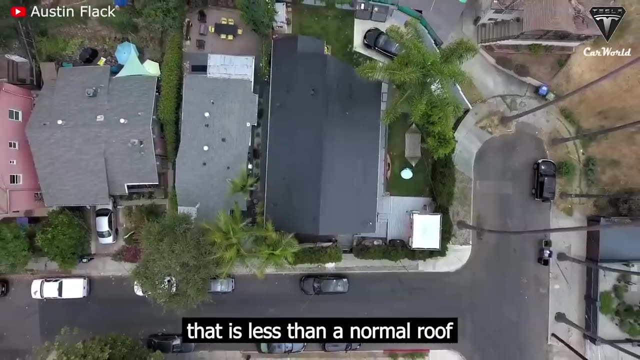 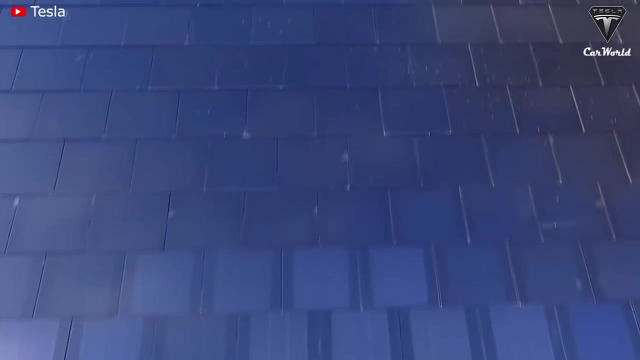 And it's not just solar energy. It's solar energy. And with that being said, Tesla also made a big splash with a new solar roof. Unlike Tesla's other offering of solar panels, these tiles are made to look like normal roofing shingles. 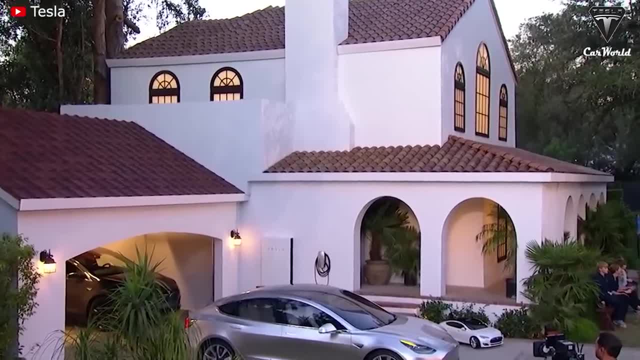 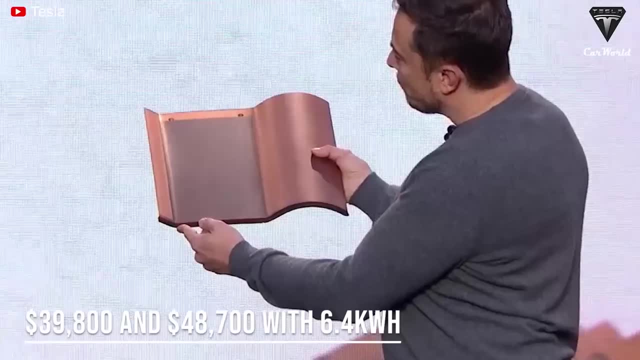 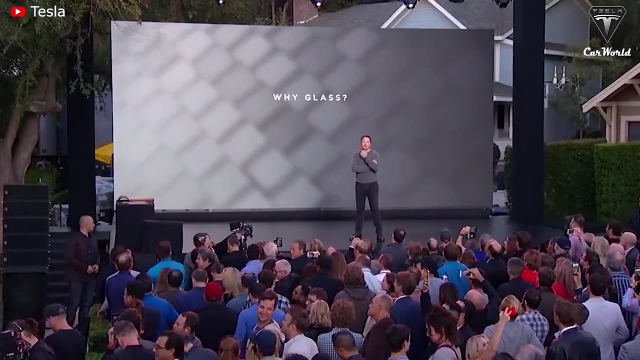 electricity for your home. A Tesla solar roof comes at a significant cost, however- between $39,800 and $48,700, with 6.4 kilowatt hours, and potential buyers might wonder how long it might take for the resulting energy savings to break even. The solar roof provides 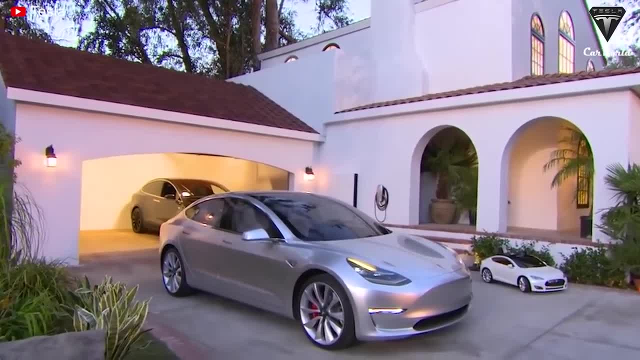 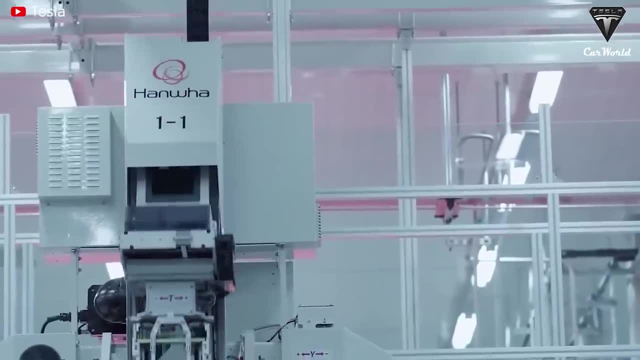 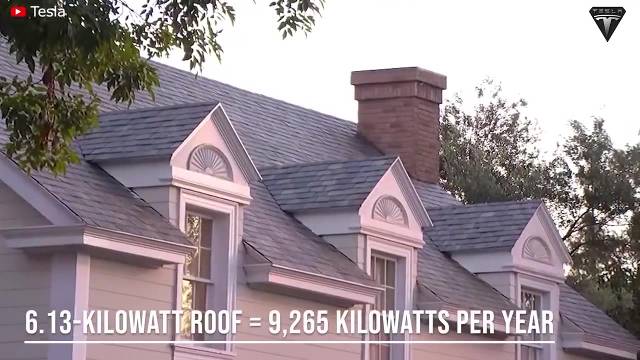 clean and green energy without any emissions, making it an intriguing choice for homeowners looking to reduce or even eliminate their power bills. Using an example of a 2,000-square-foot home in California with a monthly electric bill of $150,, Tesla recommends a 6.13-kilowatt roof. 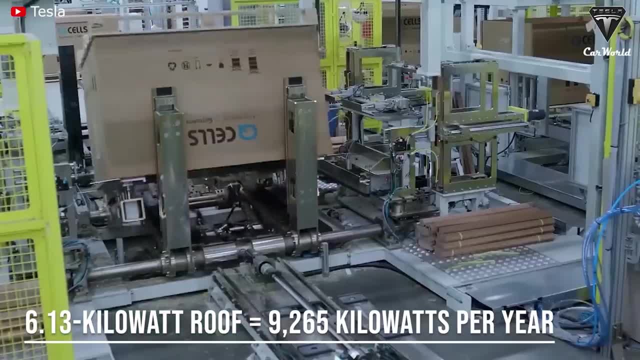 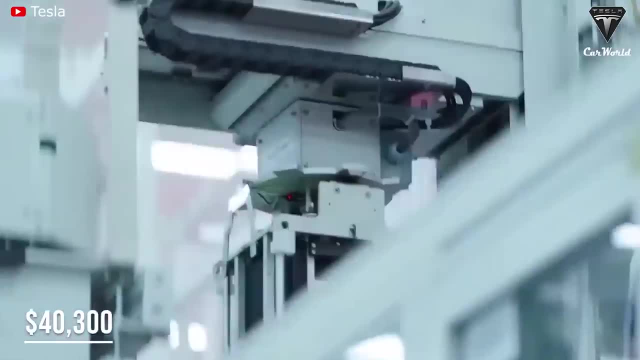 to provide 9,265 kilowatts of power each year. The cost of a new solar roof at this size, including installation, is $40,300.. Since the old roof has to be removed, there is a $6,800 charge for roof tearage. Moreover, with the Powerwall system maximizing the potential power savings, buyers will be first set back by another $11,000.. Federal and local tax incentives will lower the cost by $13,600.. For this example, a roof could cost a total of $45,500, including installation. 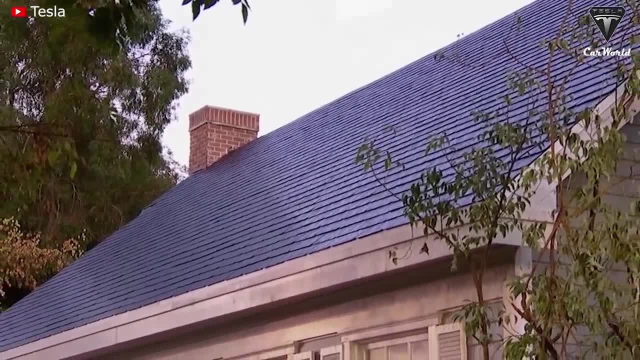 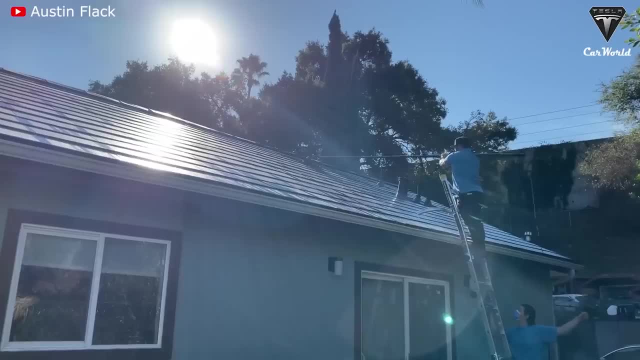 Moreover, Austin Energy's value of solar tariff pays you a little under $1,000. This means that the cost of a solar roof can be a little under $10 for every kilowatt hour your solar panels can generate. Dividing the total price of $44,500 by the $150 utility bill results in the total cost. 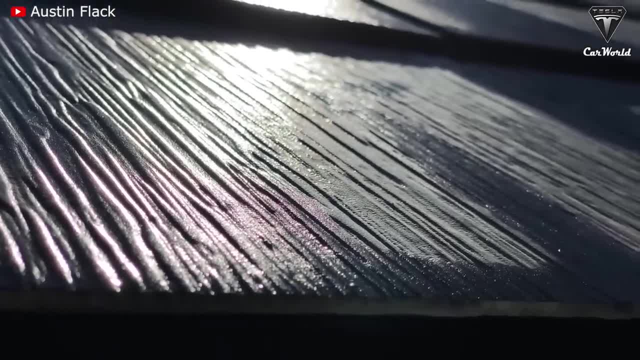 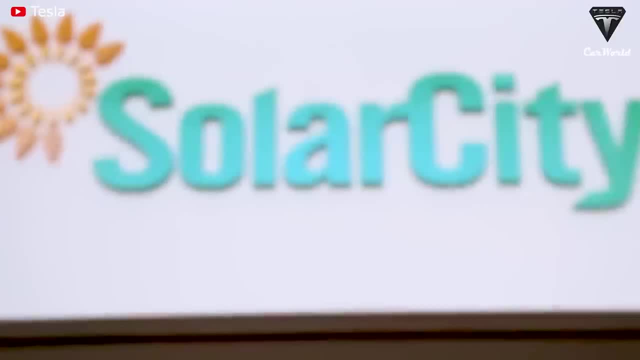 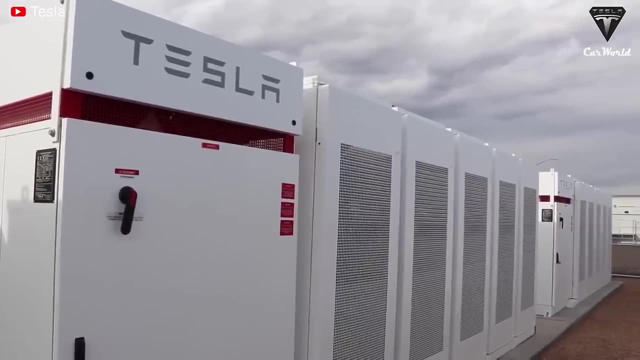 of the investment being recovered in 297 months, which is 24 years and 9 months. While a Tesla solar roof is definitely a long-term investment, it comes with plenty of benefits that can be enjoyed long before it fully pays for itself panels, but supplies and installs them. 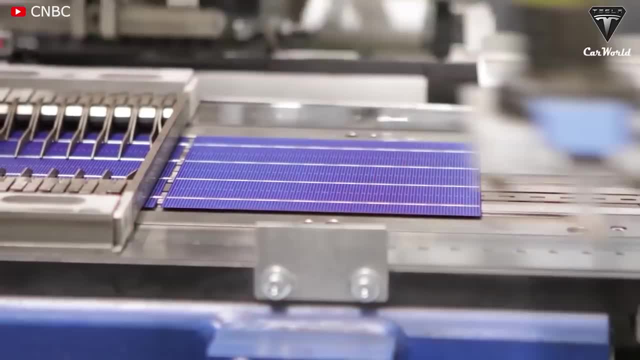 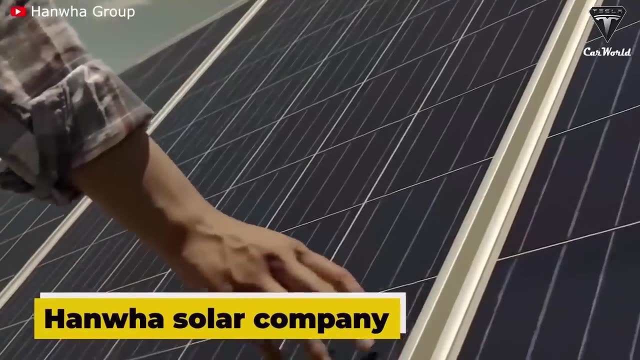 The tech giant partnered with Panasonic for a while to create its solar cells, but this partnership had ended in 2019.. Tesla is now working with a company called Hanwha to manufacture its solar panels. There has been a lot of skepticism, since they are shipped from China. 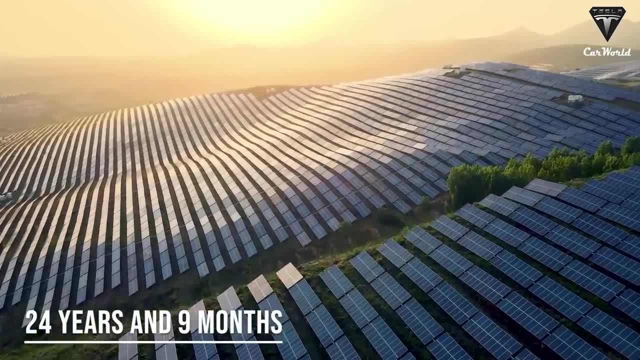 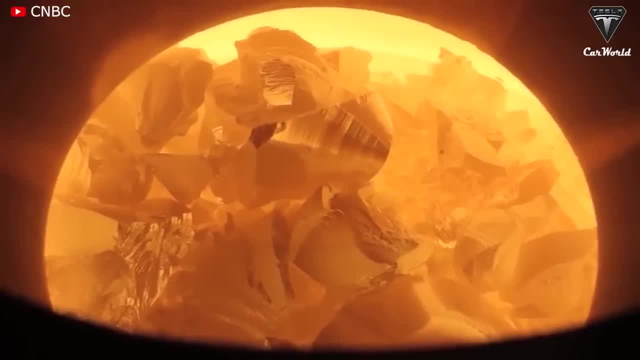 A solar panel has a useful life of about 20 years. That means a lot of panels installed in the early part of the century are ready to be replaced. But what to do with them? We still don't know how Tesla's solar panels will be recycled, but until now most 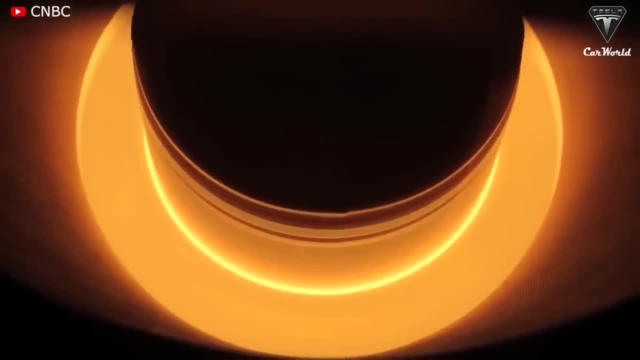 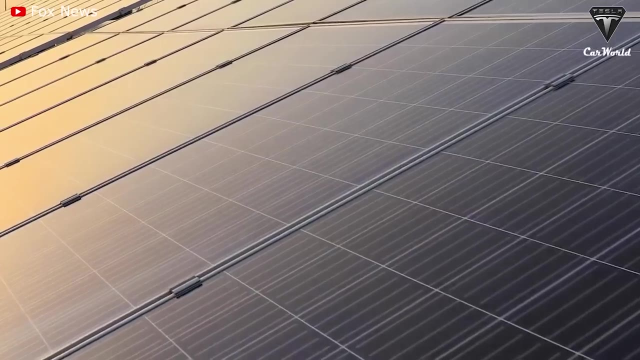 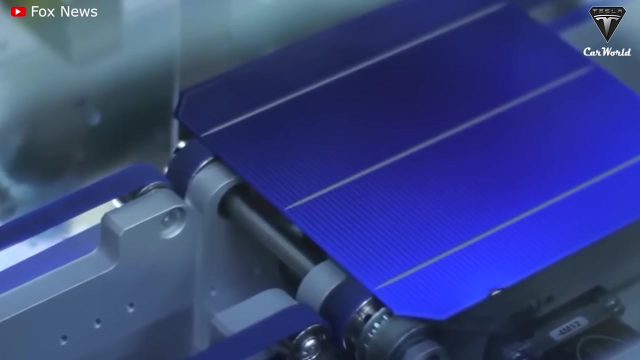 of them have been simply discarded in dumps and landfills because no commercially viable recycling process exists to recapture the precious elements inside them. There are lots of raw materials that go into a solar panel, but getting them back out is hard. The envelope-sized silicon cells inside solar panels are first separated from the sheets. 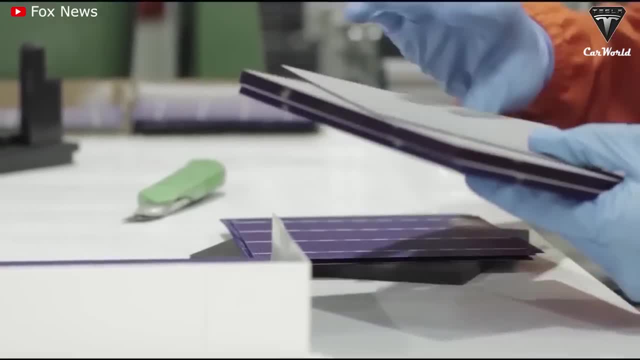 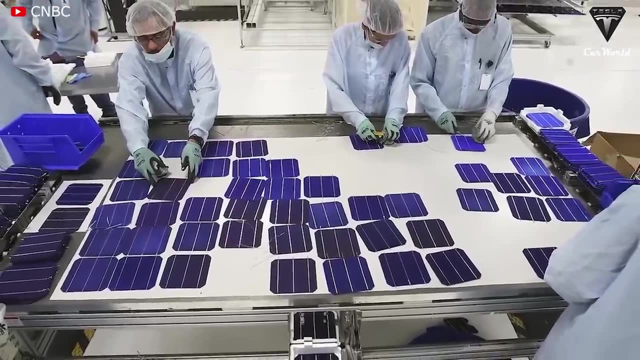 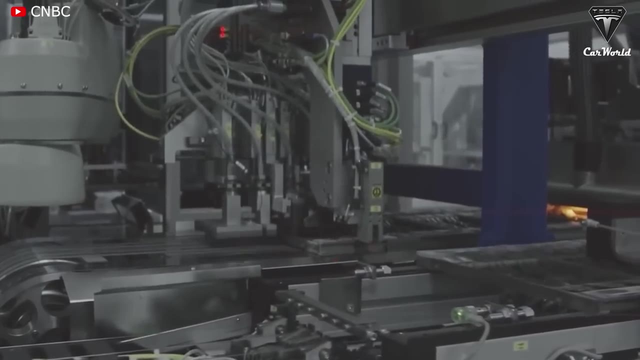 of polymers and glass surrounding them using a hot steel blade, While the recycling process uses harsh chemicals by recovering lead, the process has also the potential to eliminate an environmental hazard that would otherwise wind up as recycling waste or in landfills. There is potential to recover about $15 worth of silver from each panel, but there is no. 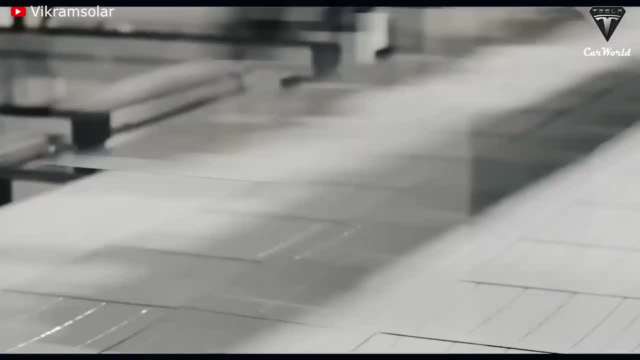 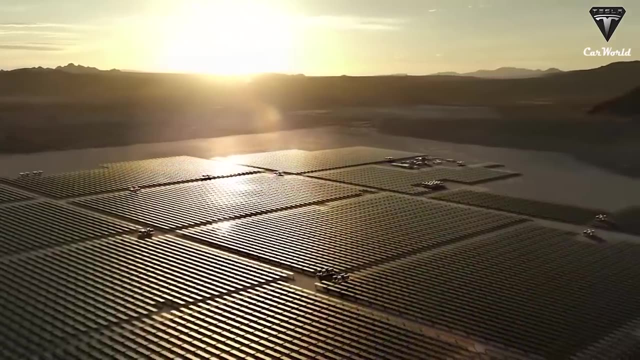 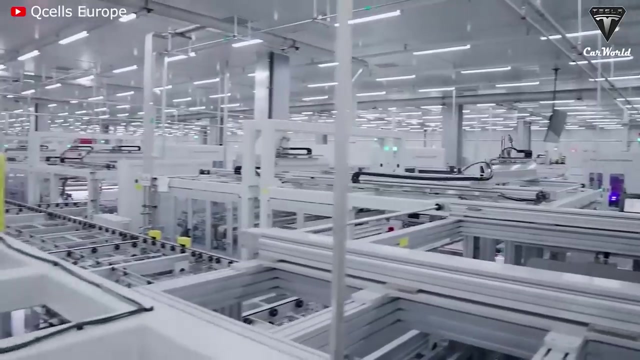 way yet to reclaim the silicon without using an expensive and energy-intensive process. Tesla may be a big name, but many other companies have slowly inched up in the solar roof. There will be more to come. race GAF Energy said it was building a $100 million facility in Georgetown, Texas. that will 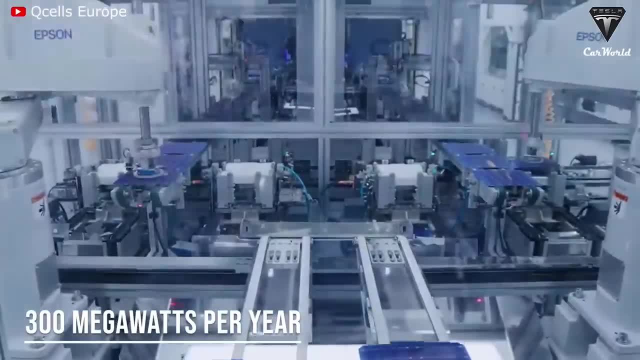 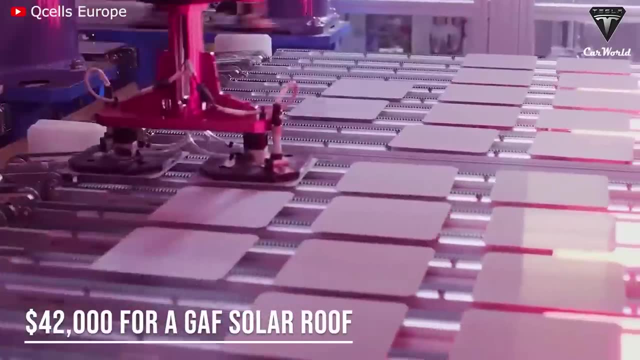 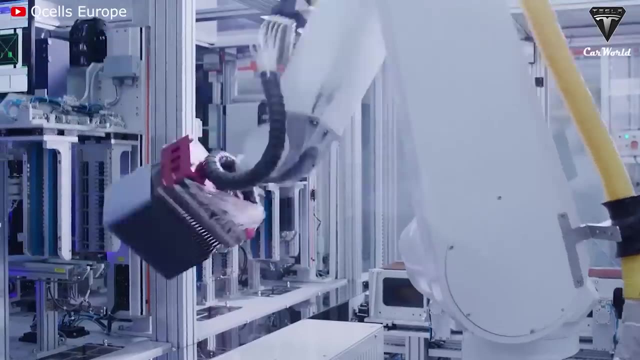 bring its domestic production capacity to 300 megawatts annually, up from 50 megawatts today. You can expect to pay around $42,000 for a GAF solar roof, and this can be reduced to around $30,000 with solar incentive programs. However, the price can change significantly depending on. 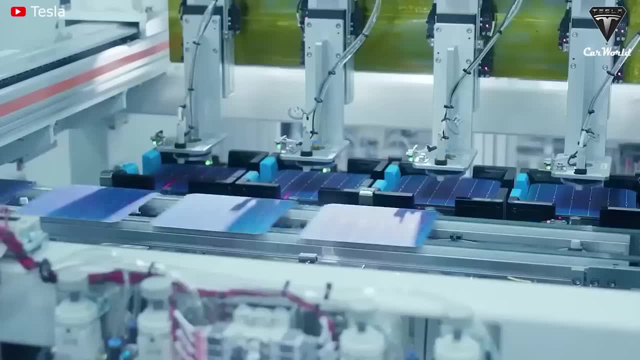 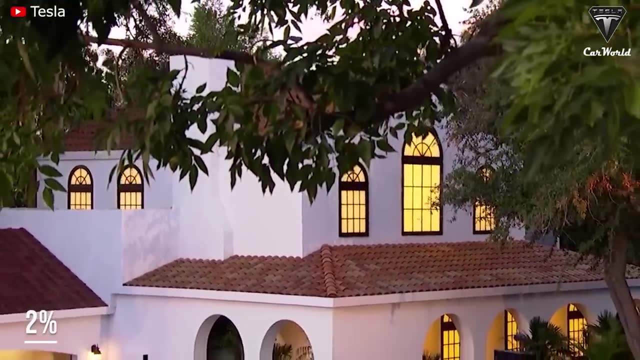 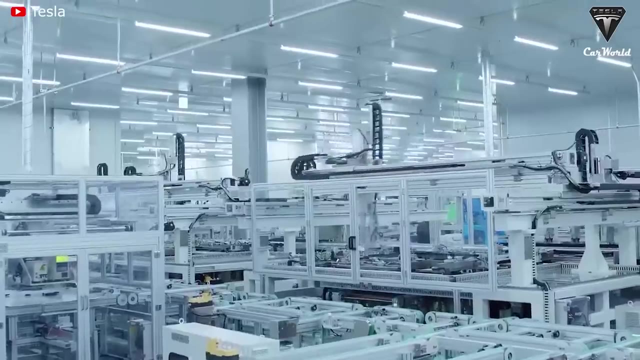 roof size and complexity. Their power production warranty offers 84.8% of initial output after 25 years of use, with 2% degradation during the first year of use and then only 0.55% degradation per year. Sunrun is now one of the leading solar installers in the United States. A professionally 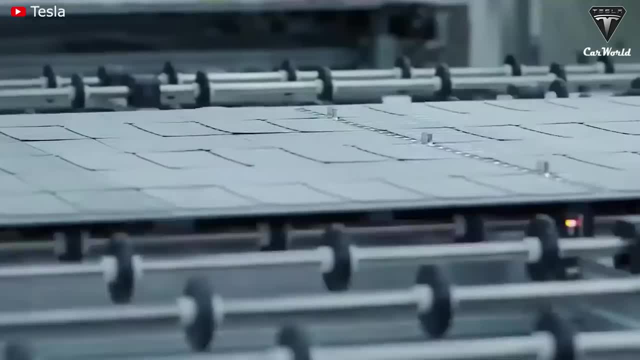 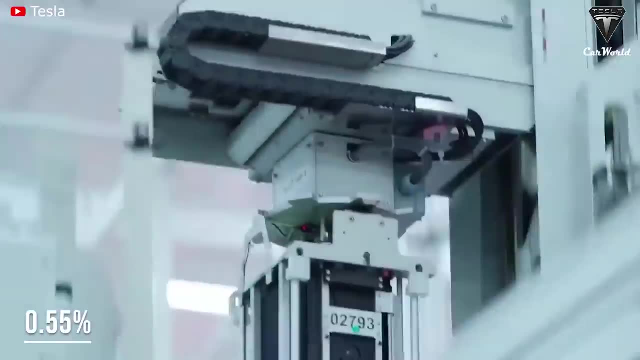 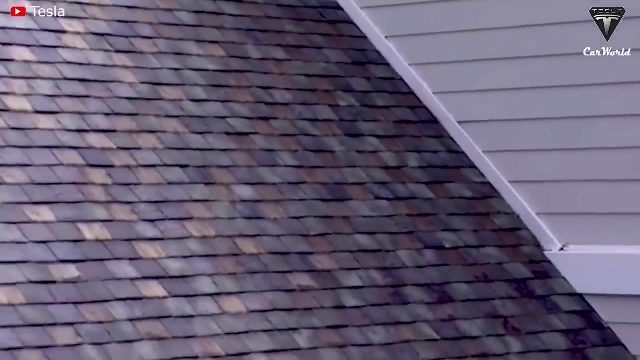 installed Sunrun solar PV or photovoltaic system, which is just another fancy way to say solar, would cost around $22,000 to $33,000.. All of Sunrun's solar panels are covered by a 10-year warranty. Although Tesla's energy roof seems to be more expensive, it has a high aesthetic value.